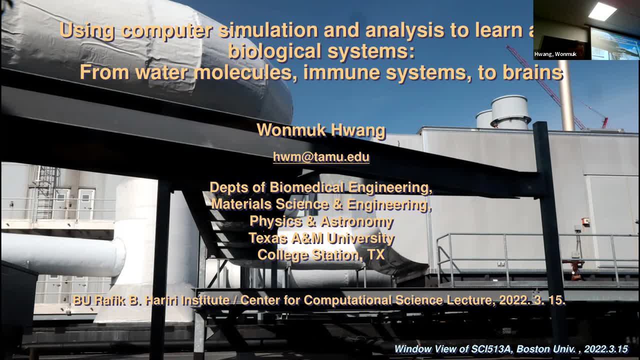 phd from the physics department- uh, working on, i guess, condensed matter theory, and so maybe he'll say a few words about exactly what he worked on as a student. and then he went to mit to work with roger khan, so a very well-known mechanical engineering that were biomedical engineers. 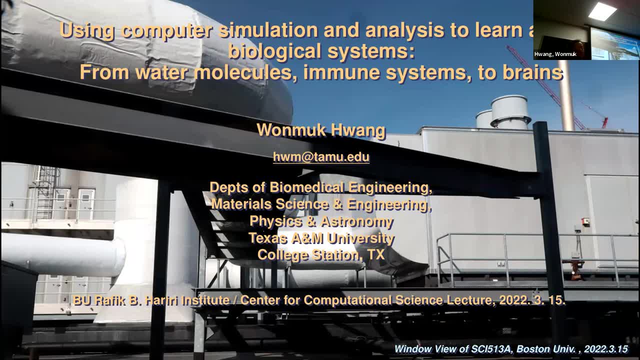 and so anyway. so, uh, you know, very interesting area, and so that's when walmart started to uh look at biomolecules, right? so, uh and uh, you know, since then walmart has been looking at the broad ranges of problems. i guess i know him mainly, uh, you know. 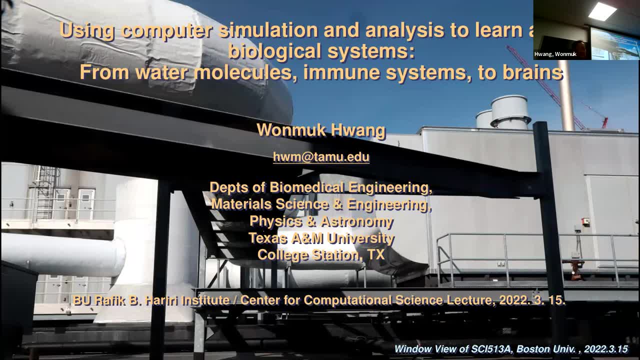 through the work of molecular motors. right, and so that's something that we have been interested in as well. but, as you can see from his title, right so, uh, we're gonna go to pretty large land scales as well. right, so, all the way to the brain, and so i look forward to, you know, uh, the talk. 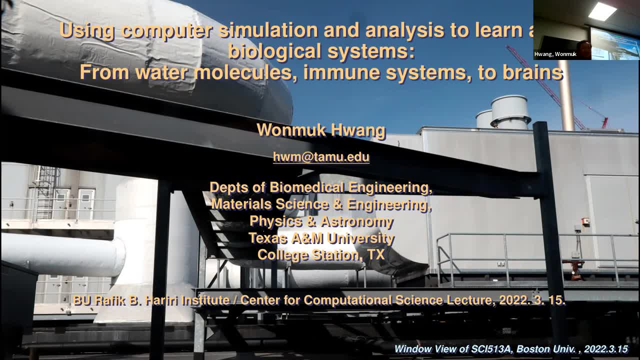 and the visit. again, you know i encourage you guys to go and talk to one month, and so you know we clearly uh has broad interest and, uh, you know, a lot of different expertise, uh and, as i sort of mentioned to some of my group members, right in addition to science, right, and so one might just 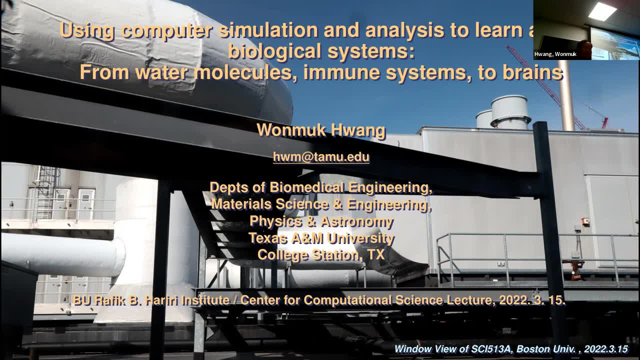 also other interesting uh, um, i guess, expertise, uh, you know, you can ask him about, uh, how to run marathon, uh, effectively, uh, in texas weather, uh, and also you can talk to him about, uh, classic korean music, as i understand it. so anyway, so without further ado, please. 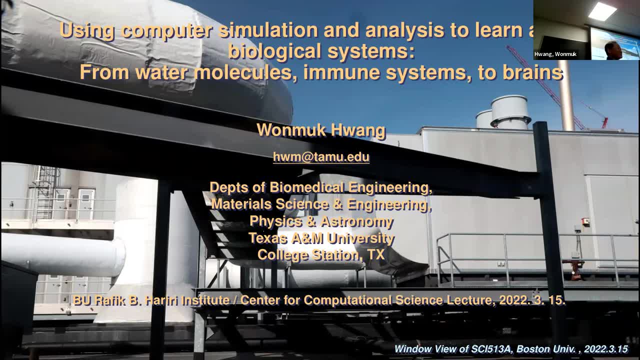 well, thanks a lot for invitation and it's a great pleasure to be back again. yeah, as a time introduced, i was a physics assistant, uh, doing contest matter theory. so at the time i had no idea about biomolecules and i didn't know what amino acids were and so on. so, uh, but uh, unless matter theory is. 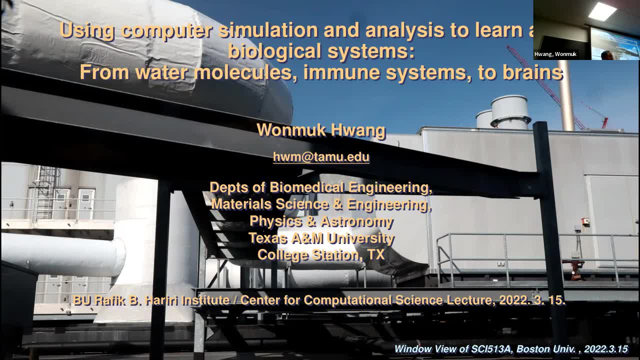 uh about these complex systems and like, uh yeah, self-organization and so on. i mean those all reflect what uh biology does. so there was actually a connection deep uh inside and i was, uh yeah, i was saying to this uh office and this morning baby said there's only like roof. so i took a picture. 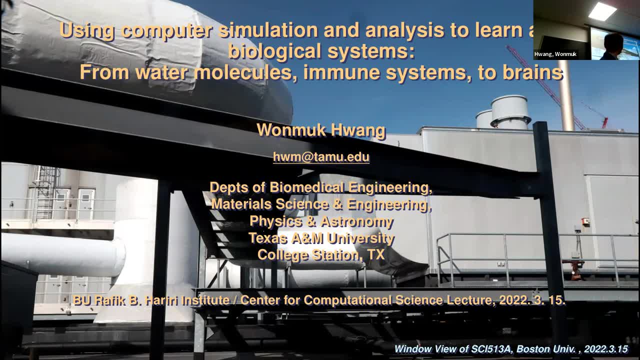 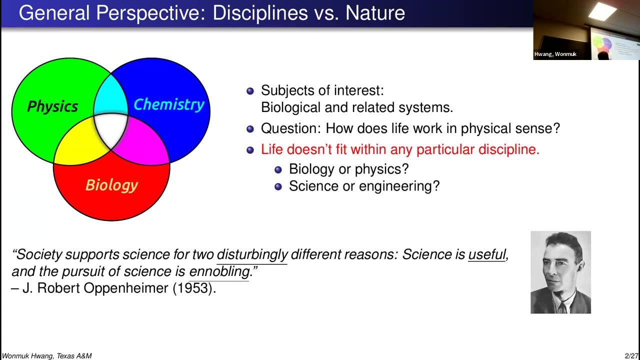 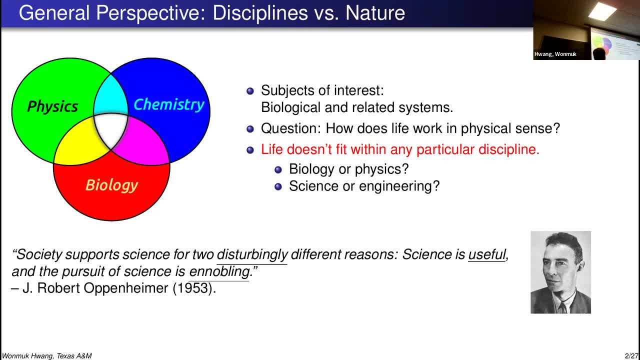 now, uh, yeah, there is almost no barrier across this disciplines and because i'm in an engineering department, or many people actually don't know or understand what i'm doing. oh yeah, yeah, that's true. so, yeah, the thing is the biological systems, life, there is no single. 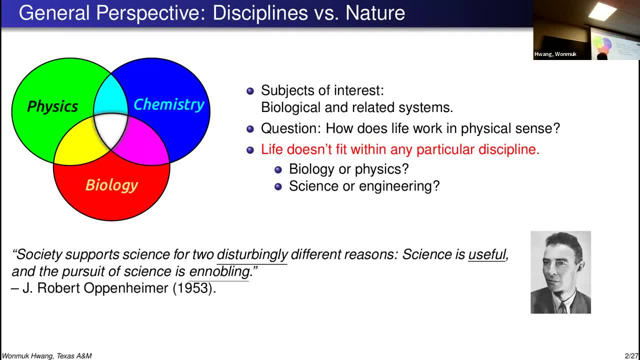 discipline that can like fit here. so we are just trying to understand this from different perspectives. and these disciplines are built mainly as like- uh yeah, human, uh, social activities. so when we study this, we have to break all the barriers. so when we study this, we have to break all the barriers. 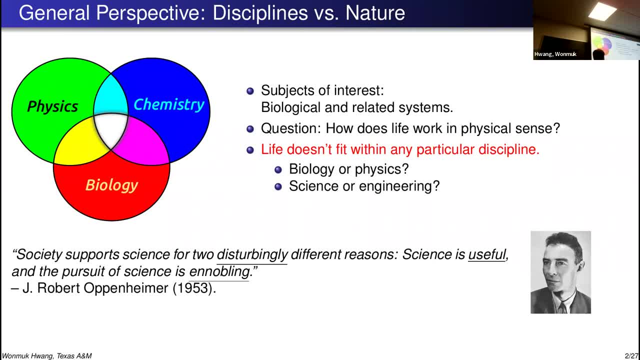 yeah, and again, because i'm in the engineering, i was telling the coach from robert oppenheimer that society supports science for two disturbingly different reasons: one is useful, the other is ennobling, and yeah, i would agree that. uh, about this usefulness and ennobling. 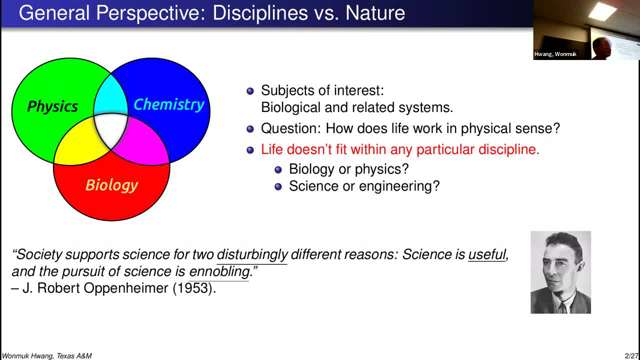 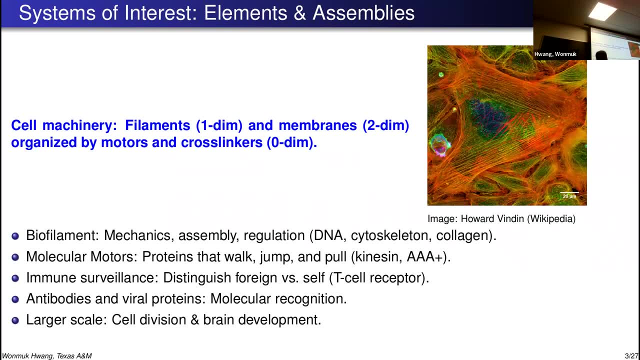 i don't know if, uh, they have to be disturbingly different. yeah, yeah, yeah, yeah. so one aspect i'm interested is mostly, like, uh, structural and mechanical. so i mean this view is from david bow's book on cell mechanics, or like describing the cellular structures as assemblies of one-dimensional filaments enclosed in compartments, membranes. 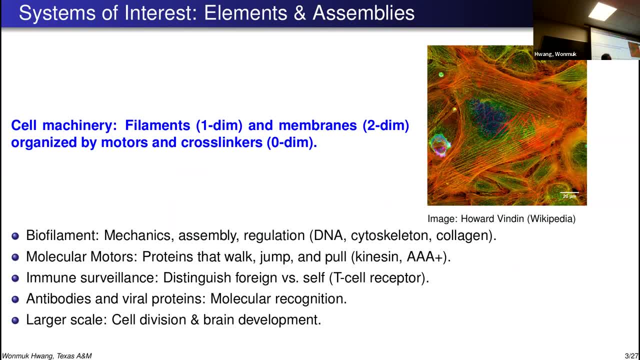 and cross-linked and moved by motors which are like zero dimensional objects. yeah, so these are the range of systems that we're going to be talking about in the next few minutes. so thank you so much. i'm interested. yeah, i will. are not going to, uh, go with like technical details, i'll just mainly focus. 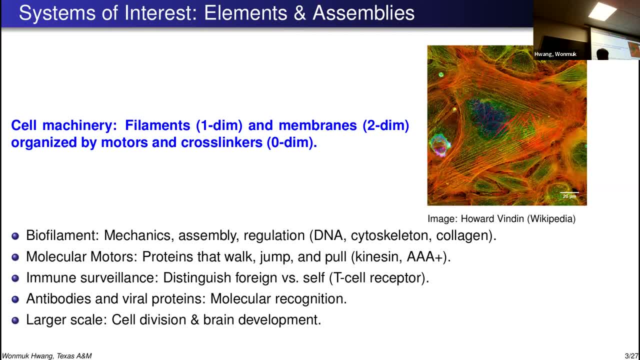 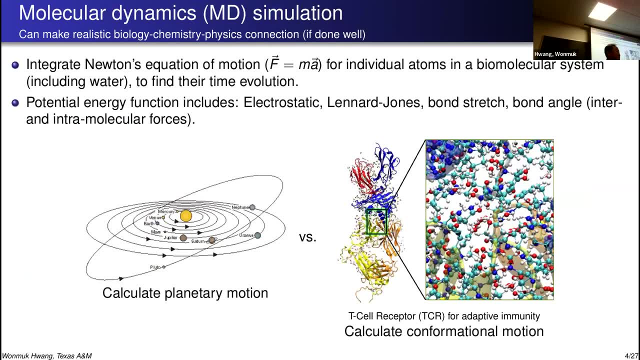 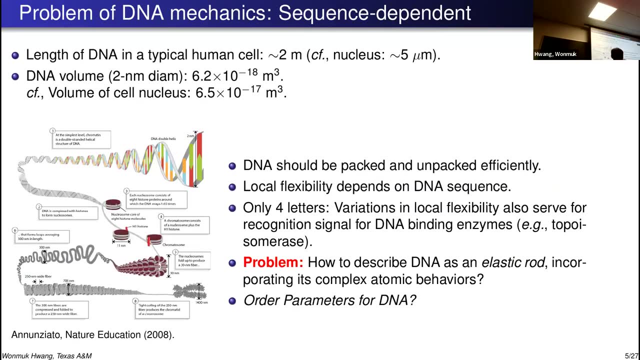 on what the problems are and what computer simulations and analysis can do about these questions. yeah, md simulation- i guess no need no introduction here. right, i'll just skip. yeah, so let's start with our dna. this is the like uh scales about dna. i mean, every cell we have has dna about two meters long. 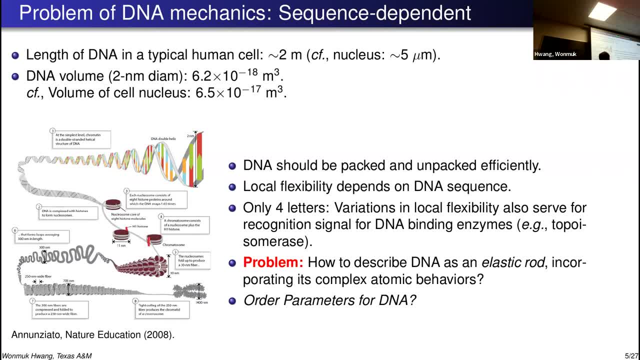 if you stretch them out, yeah, there are like uh base pairs. each base pair is like uh four angstroms long and uh they are. there are like 10 to 90 base pairs. so if you multiply it's like two meters and each dna is about two nanometers in diameter. 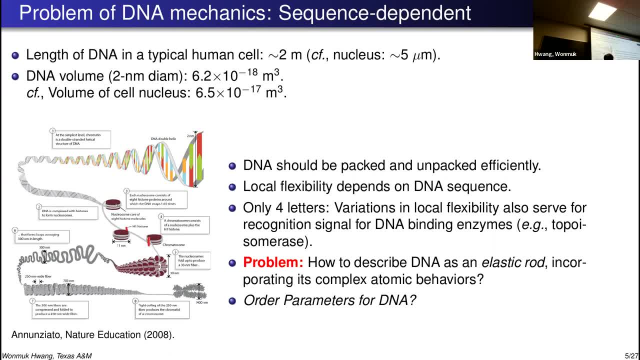 so if you just get the volume, it's about 10 percent of the nucleus volume. i mean it's not impossible. but uh, considering the dna is the most negatively charged molecule in our body, this is going to be tough. i mean the packing- so dna is packed with histones and so on- into other uh like chromosomes. 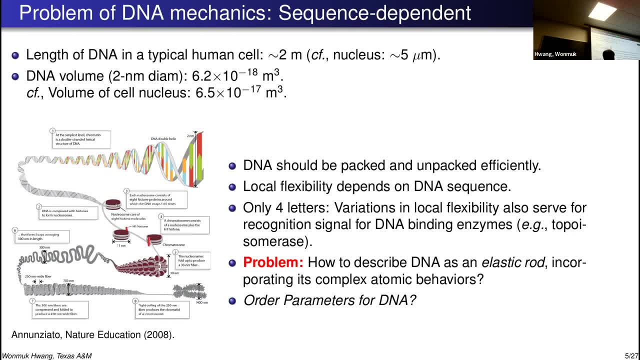 that you probably have seen. uh, but the problem is say, if you get a signal, then the signal tells us to transcribe certain genes. then you have to find where the genes are located and you have to unfold them and read the sequence and get the mrn. so this local. 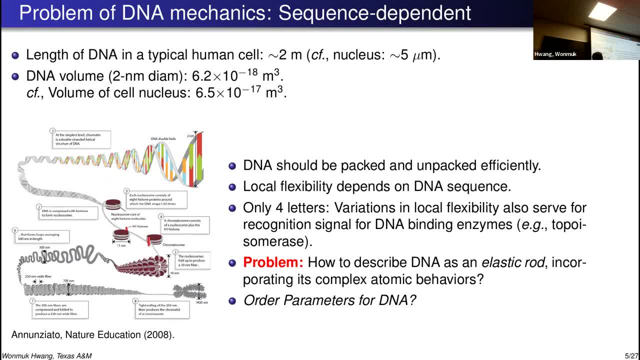 flexibility matters. and if you go to a bigger perspective, yeah, when we do polymer studies, we can try, i mean, describe polymer as a line. that's a great uh achievement, uh done by uh flory and uh design. but in biofilaments it's not just that like uh. 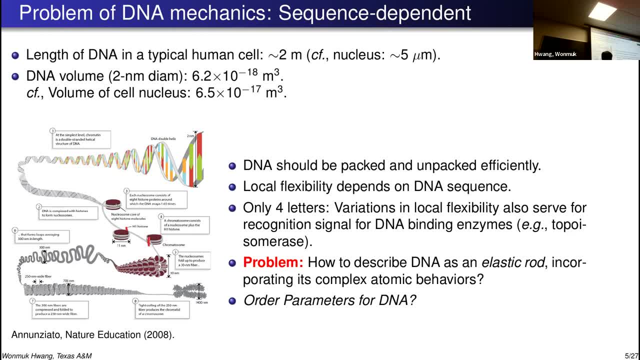 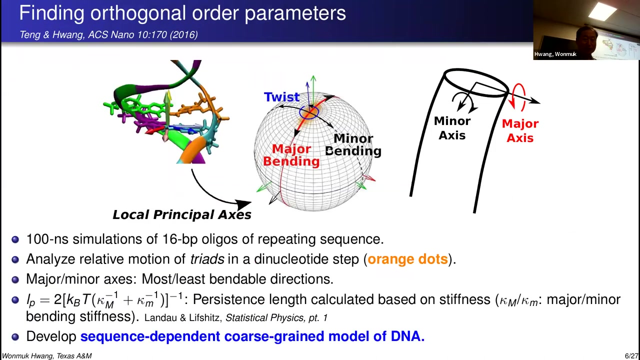 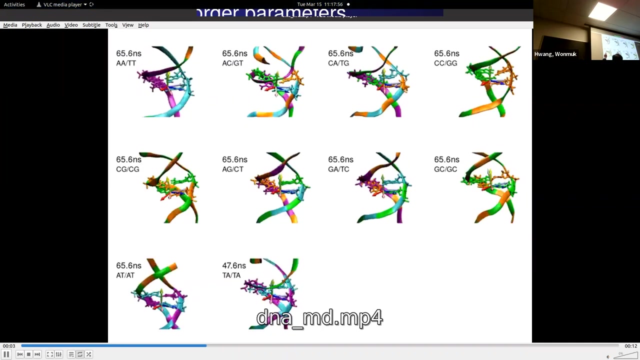 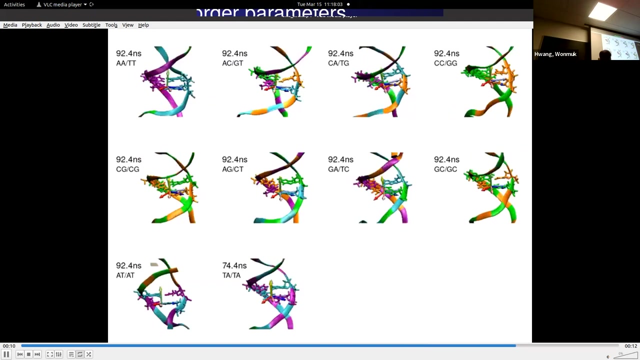 control length related behaviors, but actually the sequence matters. so where dna is more flexible and less flexible dictates how they can be transcribed, and so so the problem here is how to describe this dna. the elastic rod that reflect the sequence dependent sarà the consumption of one data. 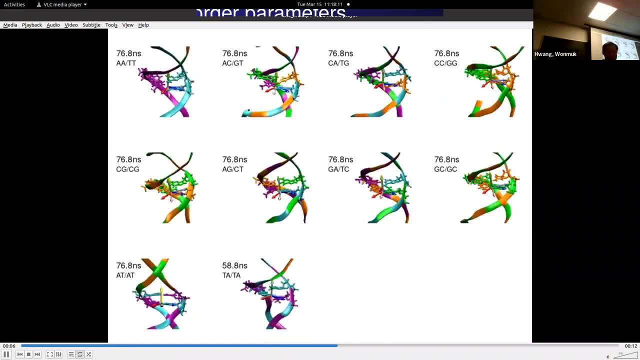 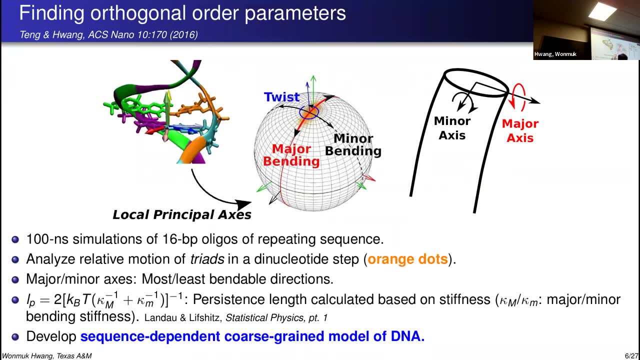 here relative to the previous one, and this is the like a sprinkled plot, or this axial vector- and you can see the orange dots- which tells how the space pair moves relative to this, then it is an ellipsoid ellipse, so there is a major bending direction and the minor bending. 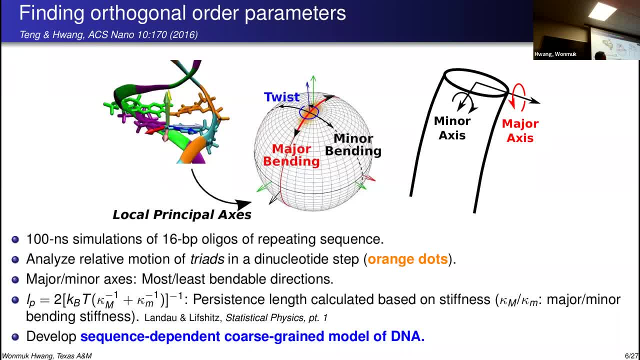 direction. it's like if you have a ruler it's easy to bend in the inner way than the transverse way. so from DNA you can find this major and minor axis. then you can apply the Inky partition theorem to get the bending stiffness. then there is a like, a study well described in Landau and Lipschitz. 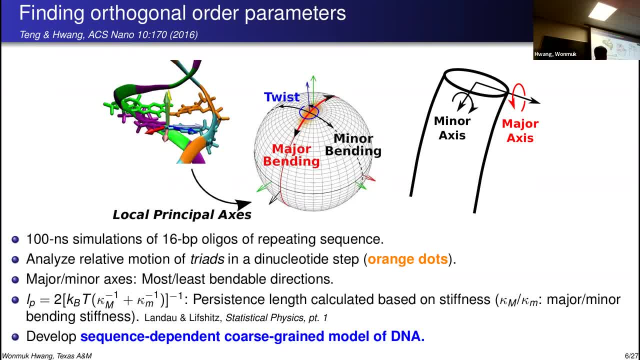 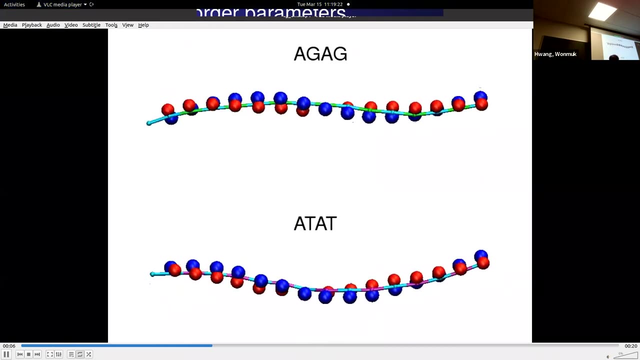 statistics committee and spoke about the persistence length of this anisotropic right here. Then you can study which space pair bends in which direction- easier or harder- and if you have that information then you can build a coarse-grained model of DNA that reflects the sequence. so this is the flexible AT-AT and this is deeper AG-AG. 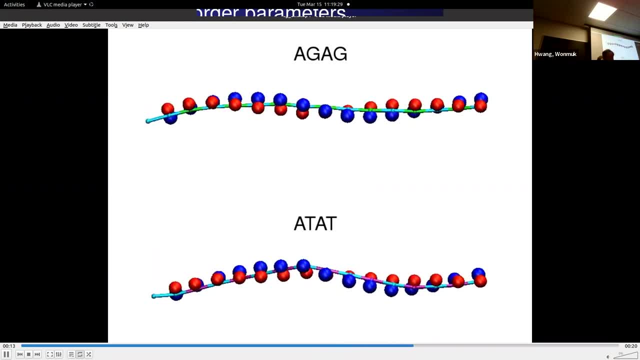 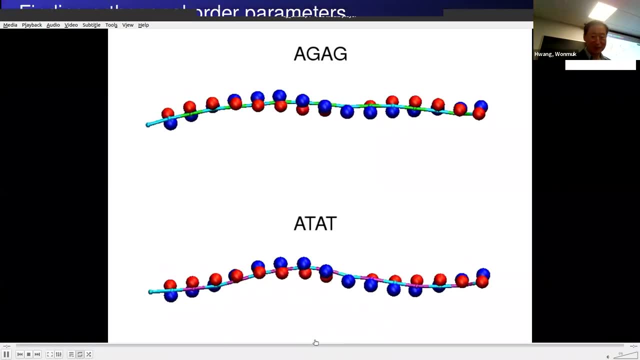 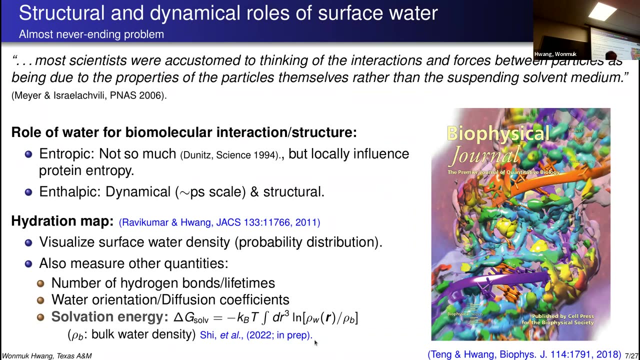 so this can be used to build up a larger scale behavior of DNA that reflect the sequence. yeah, so let's just move to the other part about the salvation of DNA or biomolecules in general. and yeah, an impressive aspect of this water is described in Israel's paper that most scientists 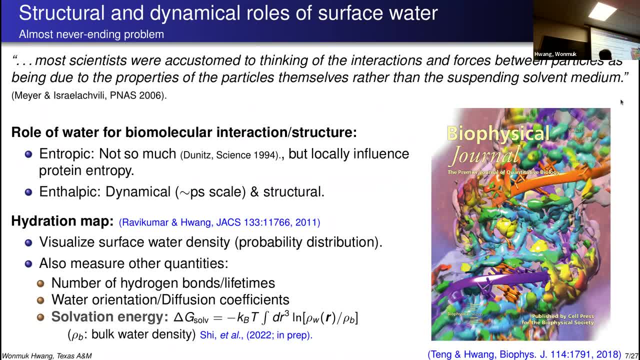 were accustomed to thinking of interactions or in forces between particles. if you have two particles- yeah, you think, how do you get the particles in the first place? yeah, you think, how do you get the particles in the second place? yeah, you think, how do you get the particles in the second place? 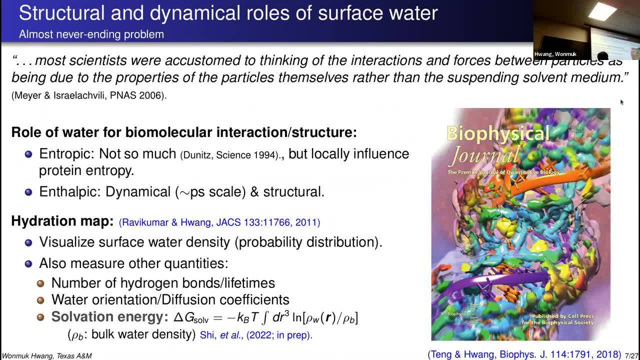 they interact with long range or like non-bonded directions, but actually the surrounding solvent medium is as important in terms of mediating their interactions. So I've been developing like a so-called the solvation map of this water, and in this case we studied the methylated DNA. 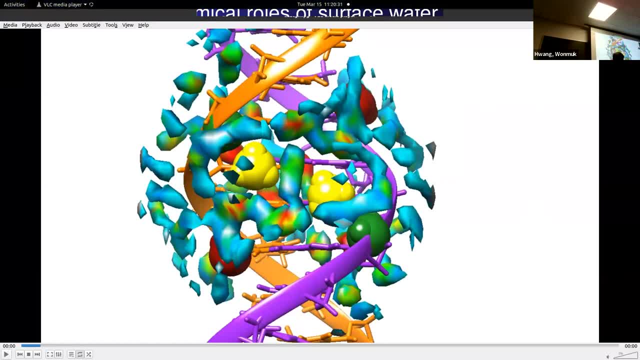 So these two spheres are methyl groups in cytosines and when our cells try to like silence certain genes, they methylate certain regions, and also cancer cells have irregular methylation pattern and so on. So there's a like interest about the methylation and these flaps are the high density water shells around DNA and there are these characteristic. 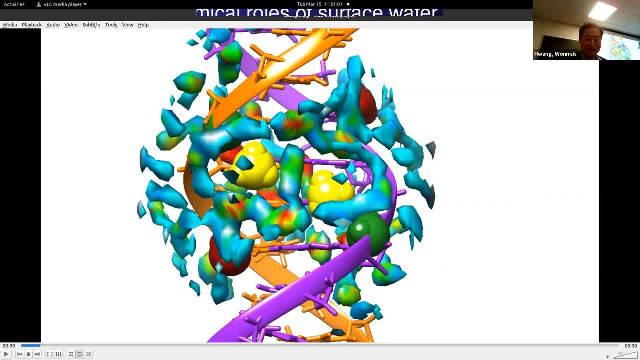 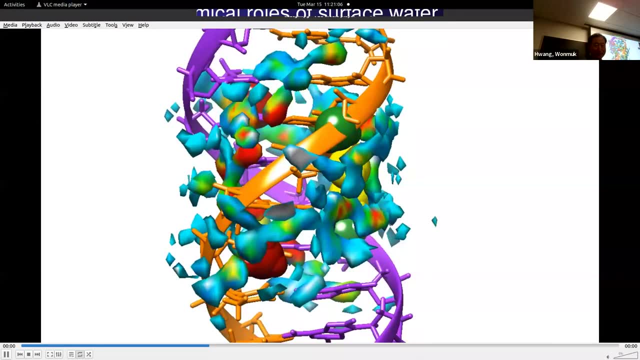 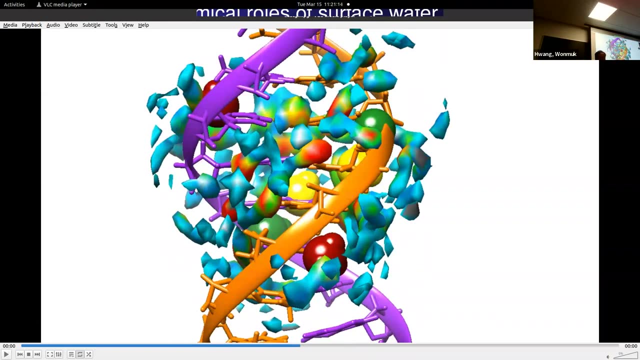 double D these and if you turn it, yeah, now we are going to the back side, the minor group, a minor group. there are deeper water molecules, so the water spine that can be seen in the crystal structure too. yeah, what's the color? the color is just a. 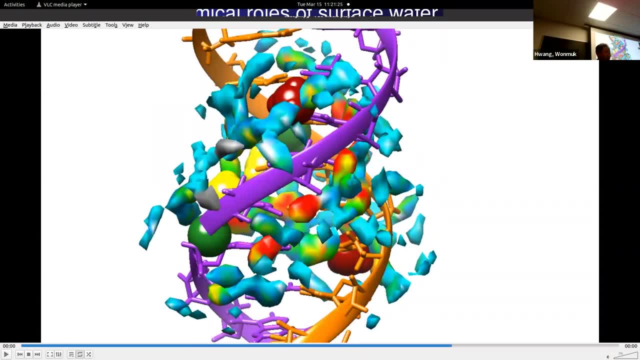 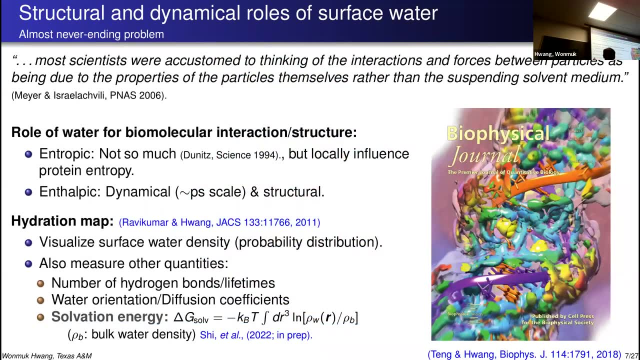 regular distance from the center, so the distance is closer. yeah, right, yeah, so we've been developing this to understand like interaction between, yeah, molecular surfaces like hydrophobic or hydrophilic and so on, and currently what we are doing is trying to get the solvation. 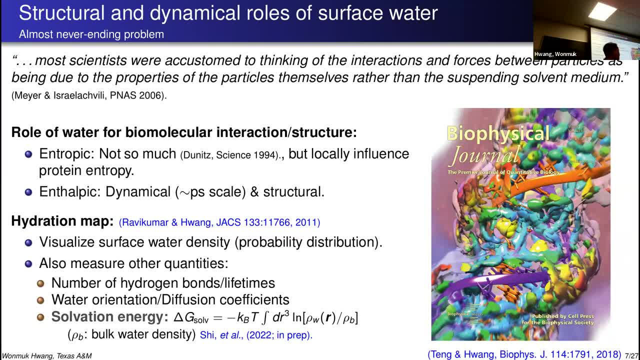 energy based on this hydration map. yeah, there are these Poisson-Boltzmann method and other types of solvation theories of continuum based and if there are, there are also the simulation-based methods and in the simulation-based methods so far people fix the DNA or for the protein. but if 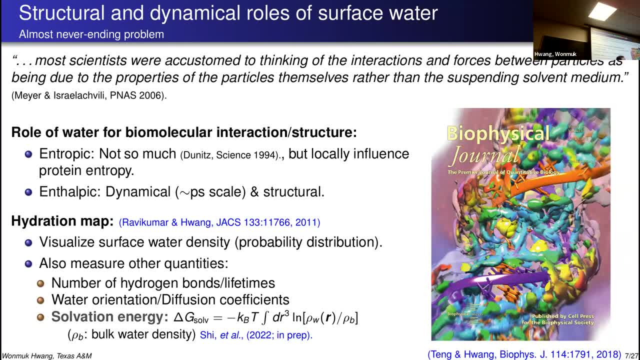 you fix, then actually, the surface hydration changes are greatly so you have to keep them moving. and since we can't calculate the density map, we can calculate the solvation energy, basically based on the density of space. in a sense, yeah, take it below, yeah, the density over the bulk density. 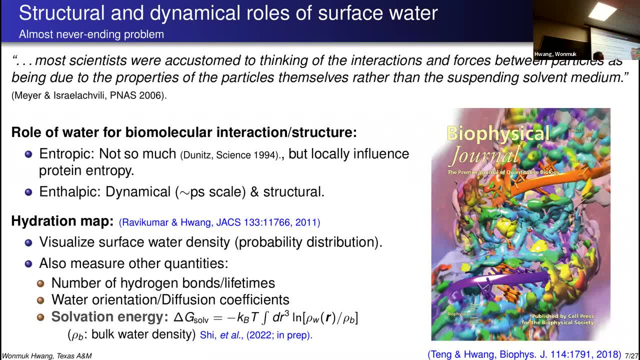 so if this is higher than the bulk, that means water likes that place. lower than the bulk, water doesn't like that place. when there are a lot of technical details of doing this for a simulation trajectory which you are like currently developing, yeah, so we moved from filament to 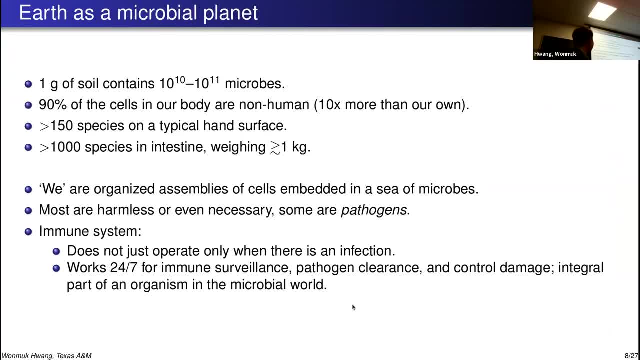 solvation, and now let's use that to understand the immune system. I'm just quickly, uh, switching topics. so there are also amazing facts about this earth. I mean, if you go look at it from distance, actually the earth is a microbial planet and we are just kind of 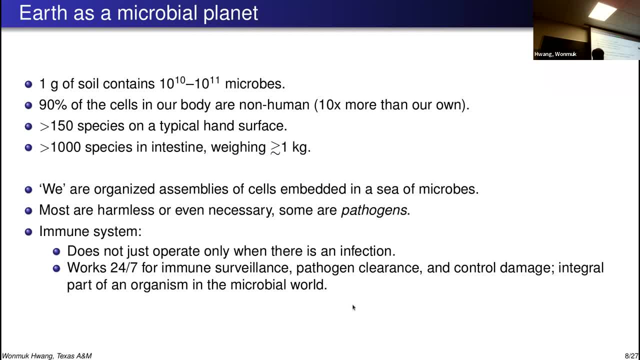 exceptions. so if you take one gram of soil, there are 10 to the 10 to 10 to the 11 microbes, and how many grams of soil the earth is is enormous. and if you just take our own body, nine percent, ninety percent of our body. 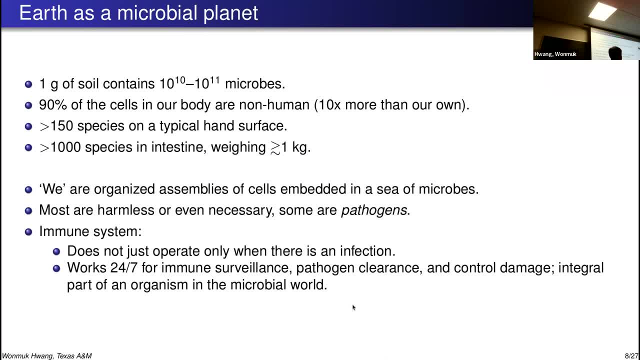 cells are non-human. they are micro microbes. yeah, ten times more than our own. if you take your palm, yeah, there are a hundred over 150 species, and in our gut, uh, there are more than a thousand species of microbes. so when we say b or i, I mean it's hard. 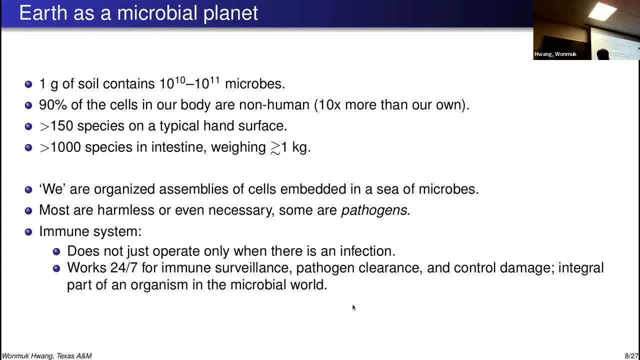 to. yeah, we are just kind of excitation is in this sea of microbes? yeah, so that tells us. I mean, we have to be interacting with them in order for to survive. and most of these microbes are obviously harmless or even they are needed for survival, but some become pathogens and 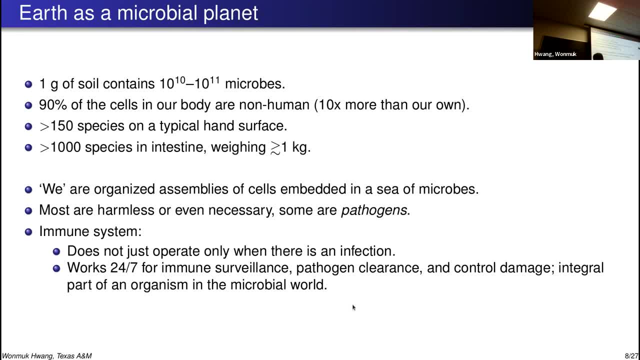 sometimes so harmless microbes can become by. so then, depending on our body condition. so this immune system or immune surveillance is constant. it's not just- uh, we think about immune response only when we are sick. it's just a basal process in the microbial form. so here are like: 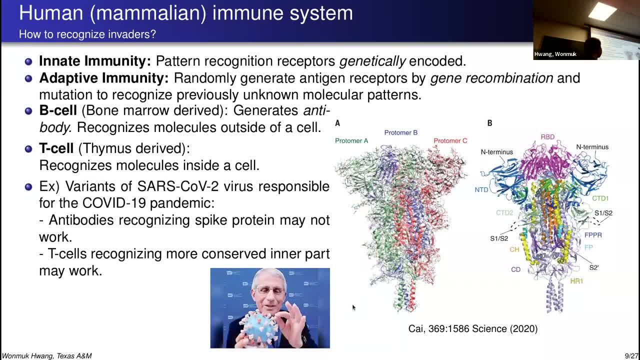 two page uh summary of the adaptive and immune health innate immune system. so we have this innate immunity where we have genetically encoded receptors that recognize, say, bacterial polysaccharides. so if you get infection we recognize those polysaccharides. then we can fight. but there are these viruses and so on. that 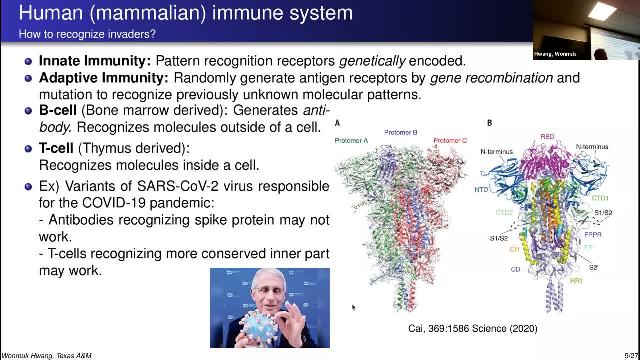 mutate, so we have to deal with that. that is, the adaptive immunity. I mean the amount to, I mean the range of these diversities tend to be like 10 or even more, oh, if you think about the exposure to microbes throughout our life. so we have to have that many of the 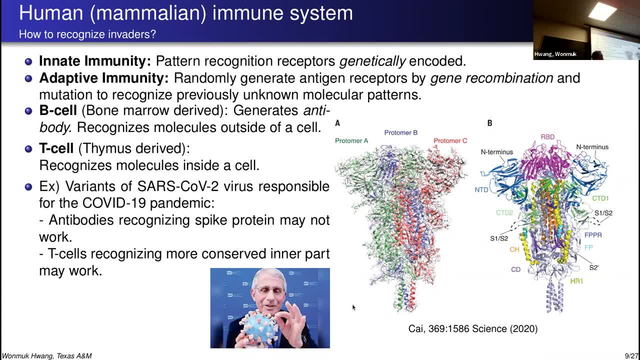 receptors and obviously we only have about billion base pairs, 10 to the 9th. so we cannot get just more than 10 to the 9th. oh yeah, if we just genetically encode all the possible receptors. so what our body does is we have gene segments and we assemble. 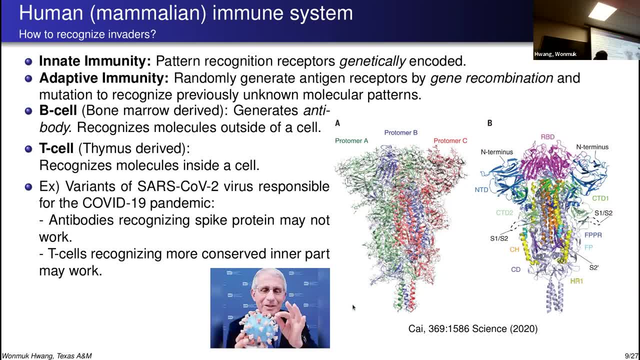 them in different combinations and also introduce mutations to generate diverse receptors. and there are bnt cells and there are bnt cells and there are bnt cells, the main adaptive immune cells. so these cells generate the antibody which we hear a lot these days due to the 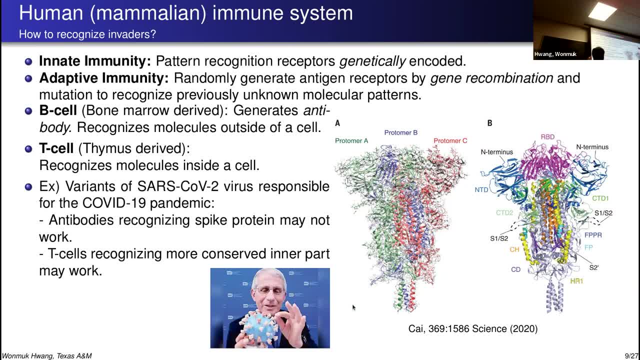 coronavirus and t cell is less well known to the public. so when we talk about antibody, I mean here's a doctor Fauci from NIAID holding this model of coronavirus. so the spike protein in the protein is this, and antibodies recognize mostly this outer surface. so when there's a variation, the 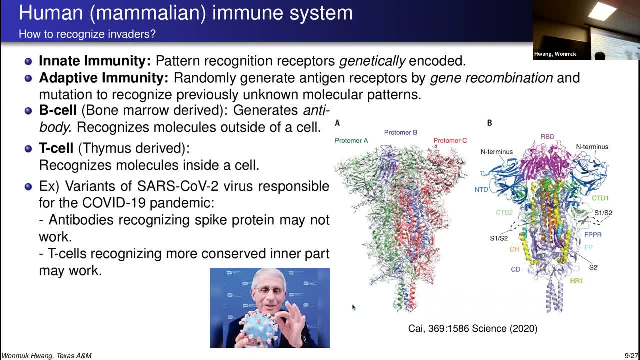 mutations. antibodies don't work well. the t cell receptors, or t cells, can recognize the inside, and inside is important for the stability of this protein. so they are less varied, because if the virus mutates inside, the stability of the spike becomes like less, then they cannot survive them. 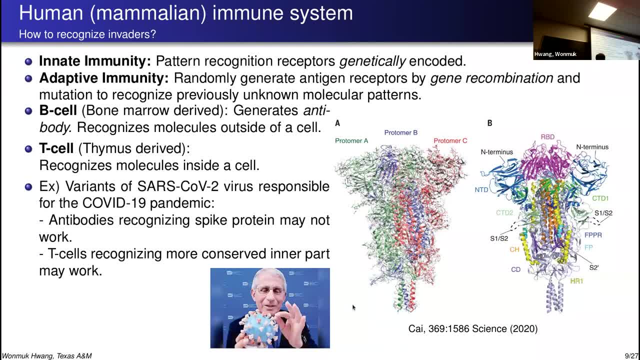 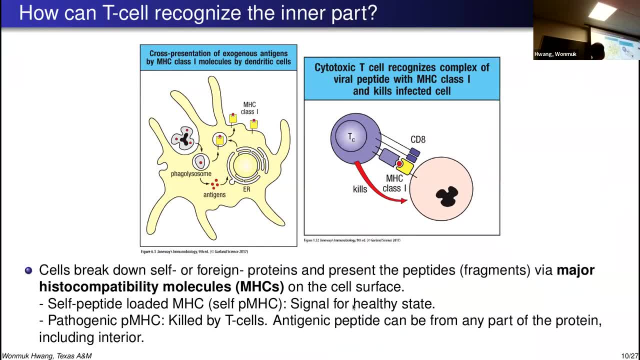 so most of the mutations are on the outside. so how does a t cell recognize the inside, as seen in a part, the next slide. and so what our cells do is we present, we like, process or chop off these proteins and present them to the surface, uh, by the molecule called the major. 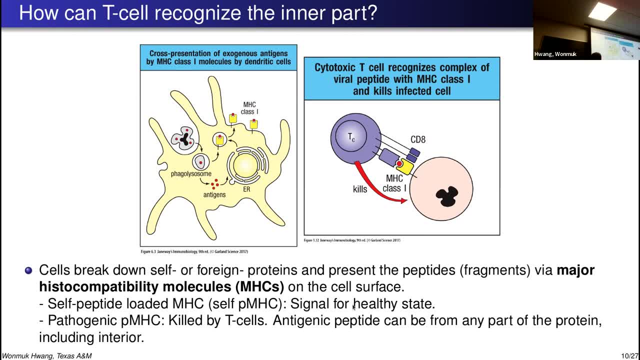 histocompatibility molecule mhc, and they are named mhc because they were the molecules are found to be like causing the graft rejection in the early days. so almost all the cells in our body have like hundreds of thousands of these mhc molecules on the surface. 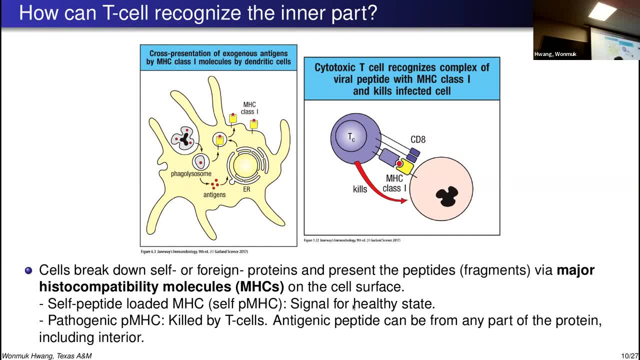 and almost all of them will hold of peptides from our own protein. I mean, we constantly process these proteins and we, yeah, when we degrade the proteins, some of the proteins end up on the surface telling them: oh, this cell is ours, so we have self. but when there are, 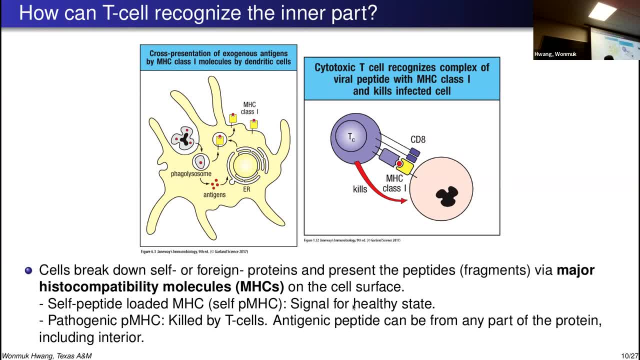 infections. some of the proteins are now displayed on the surface and we have to distinguish between self and the floor. that's the main challenge here and that's what the t cell does. and because the protein is broken down, you know, part of compound components are here, which is how the t cells can recognize. 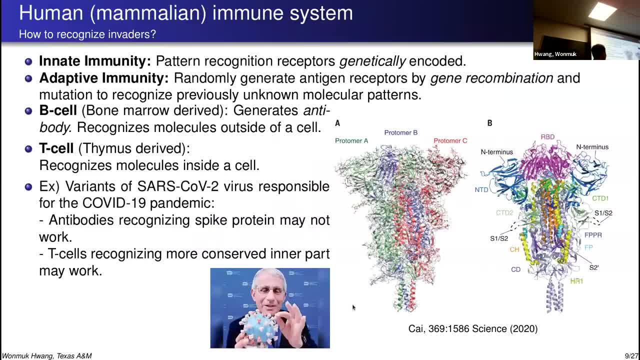 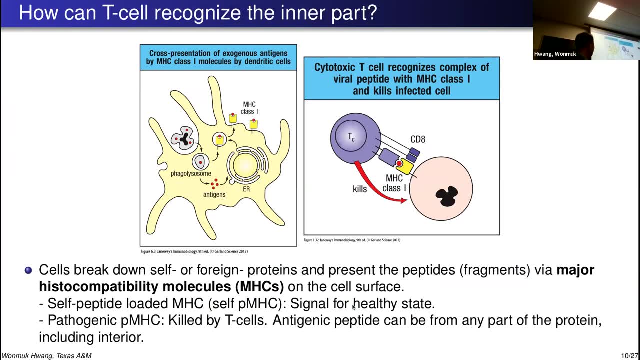 or the inner part of this protein. yeah, if you chalk this up, there are peptides generated from the inside. that's what you can recognize. so that's it in this test. oh, t cell is actually very important and when we get vaccinated, it's not just antibody, but there are t cells that are 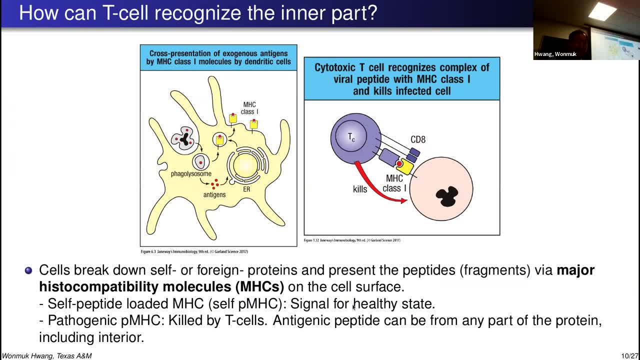 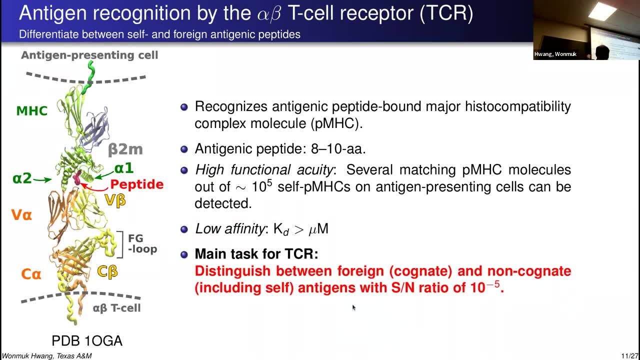 there that can recognize. uh, which is how the our vaccines work against these variants. yeah, so here's the structure of the t cell receptor and this is the dimeric t cell receptor, and this is roughly the surface of the t cell and this is the surface of any antigen. 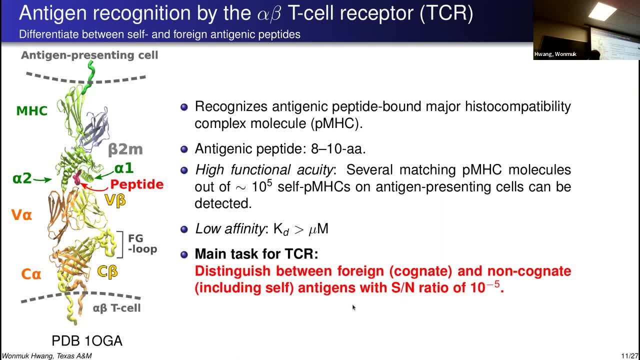 presenting cell, almost any cell, and this is the mhc structure. so you have alpha and beta, two microglial and this is the peptide held by this, two alpha illnesses. so the t cell receptor has to tell whether this is us or invader. but this peptide is only eight to ten. 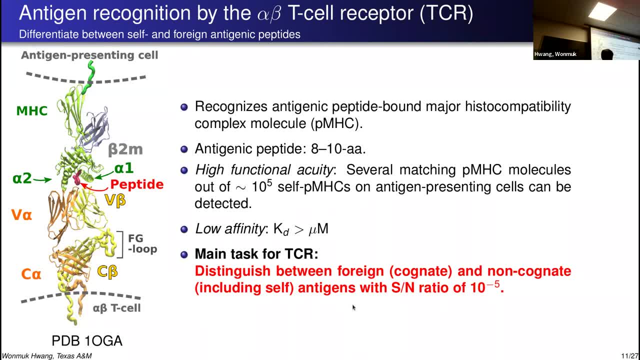 amino acids long and the t cell receptor has to be able to pick out of hundreds of thousand molecules. almost all of them have self molecules. if there are a few copies on the surface of the cell, t cell can recognize okay, that this cell is infected. so if this is infected, one in 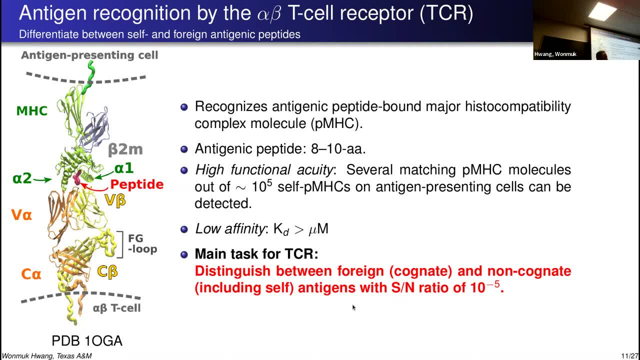 maybe a hundred thousand. there is a full impact time and the binding of it is low, greater than micromolar typically. so from biochemistry- are you all chemists here? sort of yeah, so micromolar- i mean greater than micromolar affinity- is called undruggable- it's so weak. and antibodies. 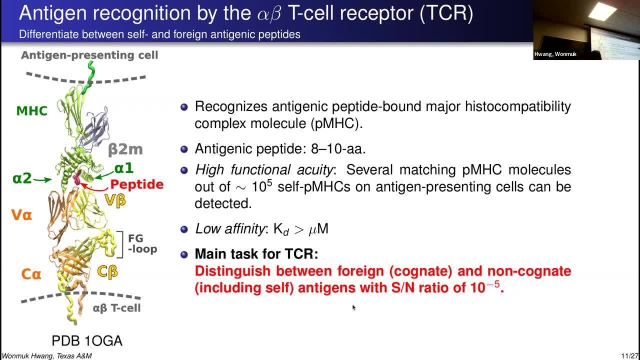 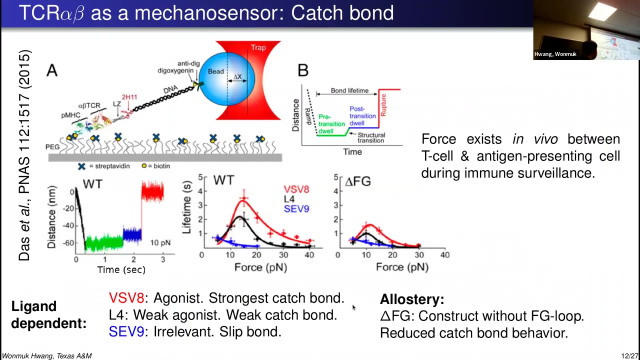 typically work down in the nanomolar range pretty strong. so how does this uh like? uh, conundrum? uh, yeah, all right, refining, but very sensitive, yeah. so this is the main test for dcr, and recently my collaborators matt lang at the vanderbilt and people 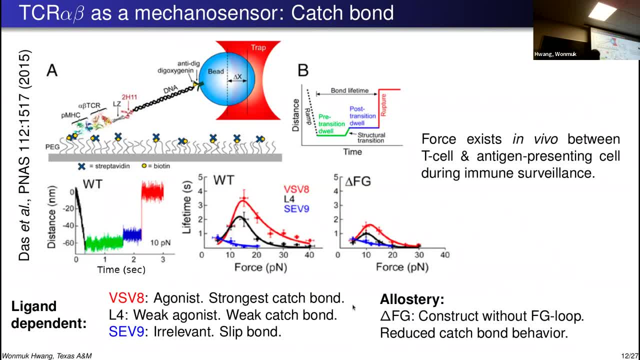 from harvard medical school. they were beginning to see one big contribution of this sensitivity, which is the catch bond or mechano sensor aspect of tcr. but this doesn't move. so, yeah, when we apply force to adhesion, yeah, like sticky tape, if you apply right, you can detach them exponential. 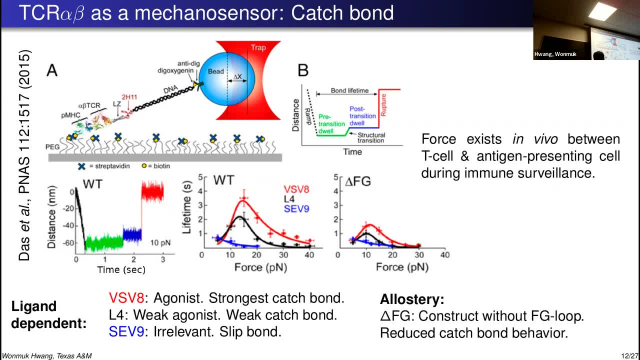 decay of one lifetime. but there are some biological contexts that increase the bond lifetime with force to some extent, and only when the force becomes great they decay. so this is called catch point. you strengthen the bond by applying force. i mean, yeah, this is uh basically uh, due to 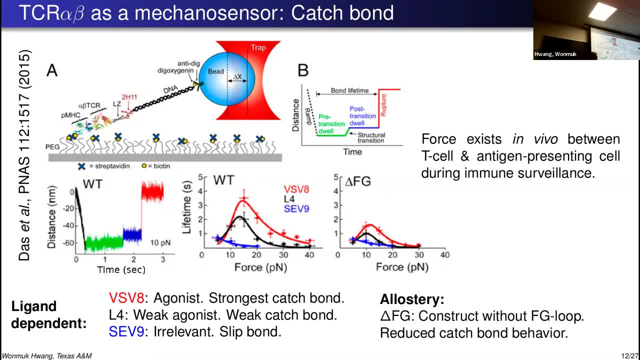 conformational change of this protein that becomes, uh like, better sticking when there's a force. and in this single molecule of assay, you know, surface has the peptide mhc molecule and here is alpha beta tcr and that's pulled by this optical track and they measure. 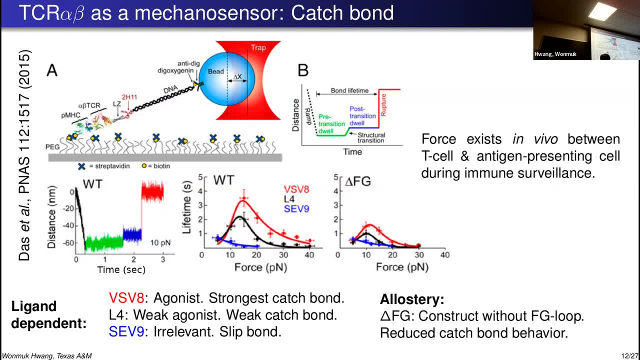 the bond lifetime and, as you can see, the sba is a vesicular somatitis virus, uh octa peptide, and that's the agonist that needs to be recognized in this system and this bond lifetime is longer. and l4 is a mutant uh like uh from valentine to use in a 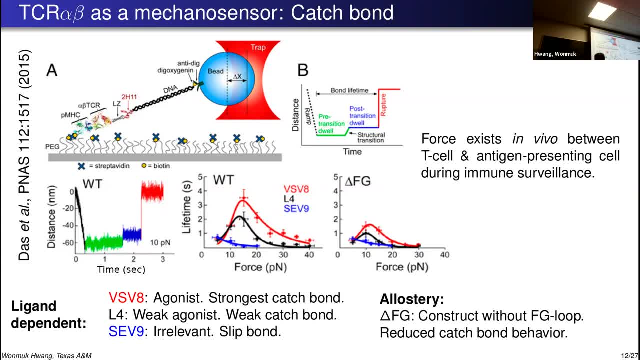 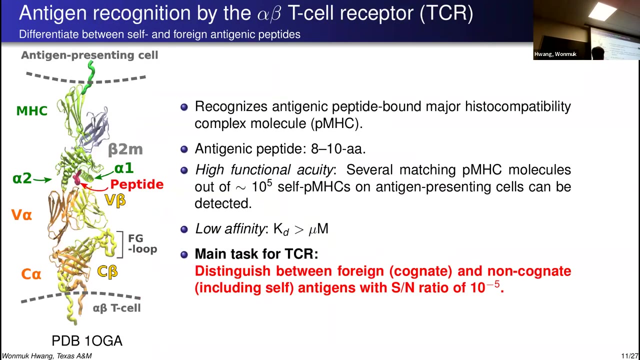 position four in this peptide. so catch one is weaker and this is the sendai virus nona peptide and it shows a slip on objective irrelevant. so this is highly dependent on what peptide is there and, moreover, they made a mutation of delta fg. so this is the fg loop, just like a. 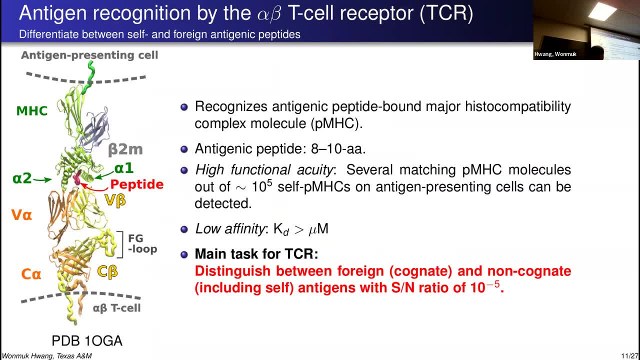 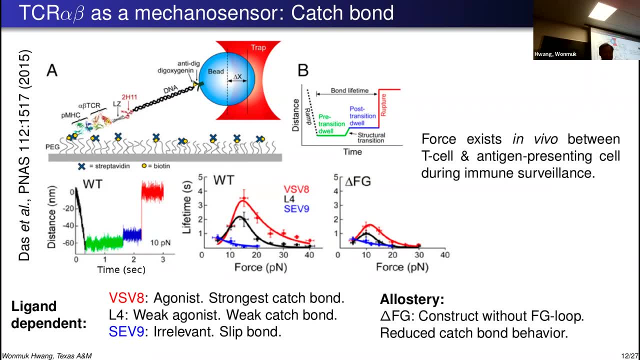 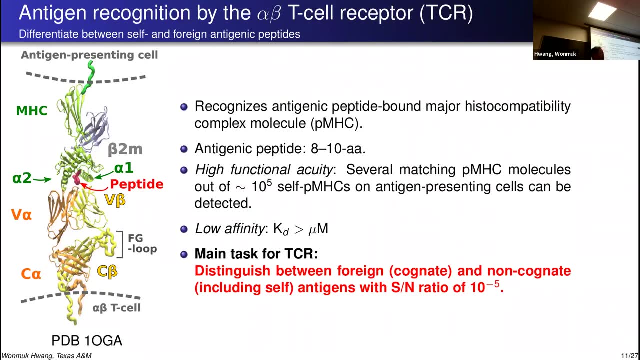 protruding elbow in this beta chain and when they deleted it they saw the suppression of catch points. and the reason why they studied: uh, the fg loop is, uh, this is like vertebrate adaptation, so if there are organisms below jawed vertebrate, so there are organisms that are. 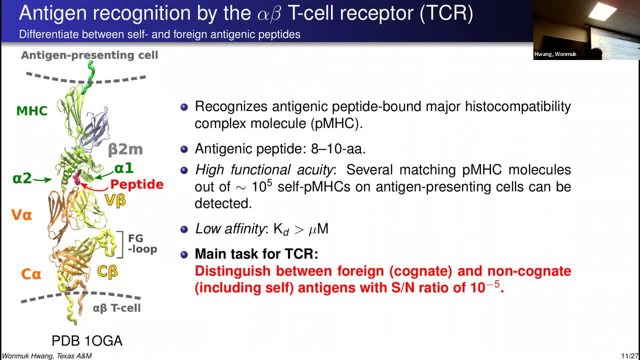 vertebrate but has have no jaws. they don't have this uh t-cell receptor. and, yeah, from jawed vertebrate that up there is an absolute loop and mammals the actual loop is the longest. so there's a clearly uh evolutionary relation. so this seems to be enhancing. 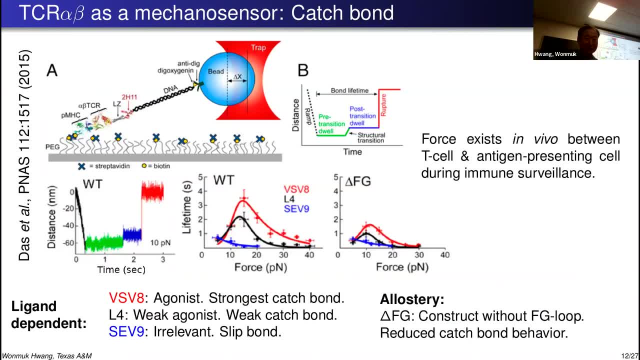 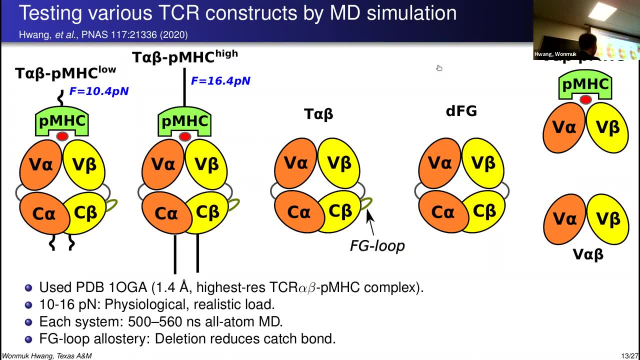 catchment behavior. so my yes study was how this actually happens from structural point of view. so i uh built a different structures with systems like the complex, the regular complex and without this peptide, mhcc, and without the fg loop to see how the behavior differs, and without 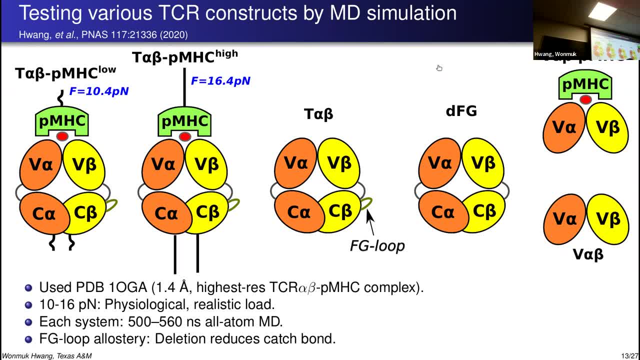 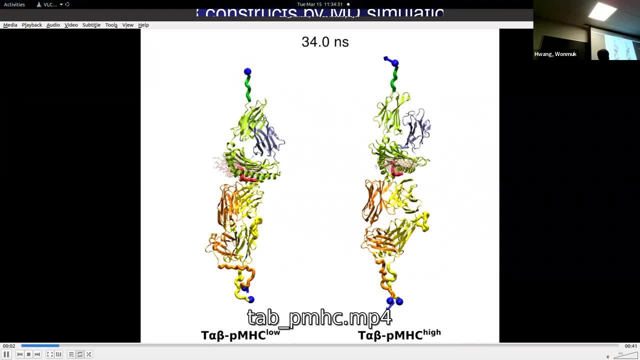 the so-called constant domain, but a peptide, mhcc, and so on. i mean, these are not the all of the uh systems i studied. there are actually more. and the simulation goes like this: yeah, you hold the ends with harmonic springs and just run it for like 500 nanoseconds. 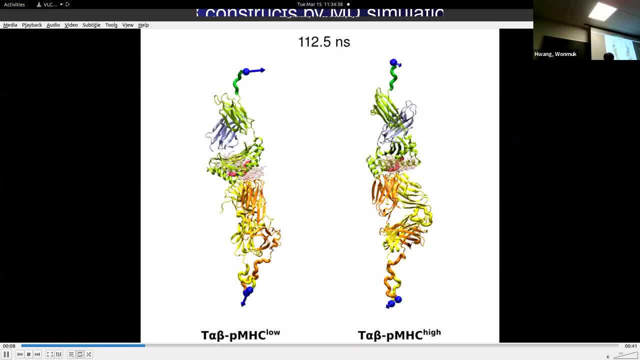 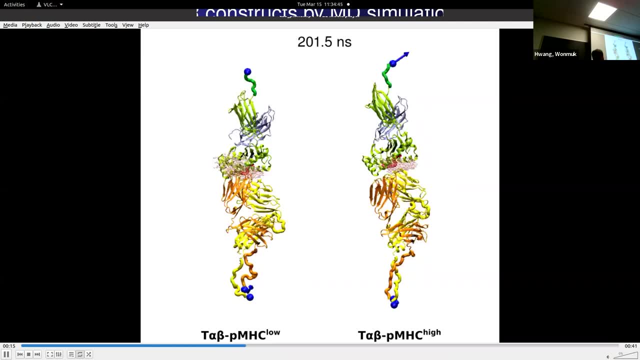 and this peak cloud is just a central mass trajectory of this peptide and, as you can see, the force factor instantaneously fluctuates. i mean there's a thermal aspect too. so this is a low extension, high extension. so when people study, uh, this adhesion or bonds between like 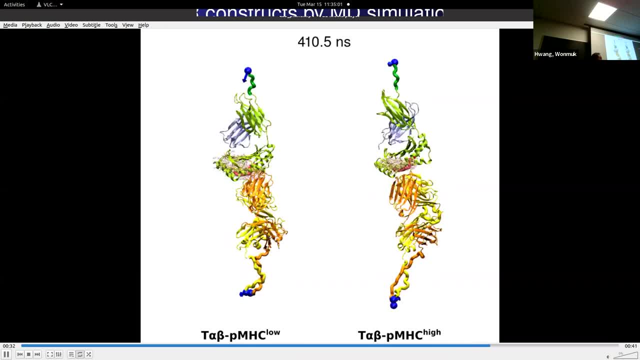 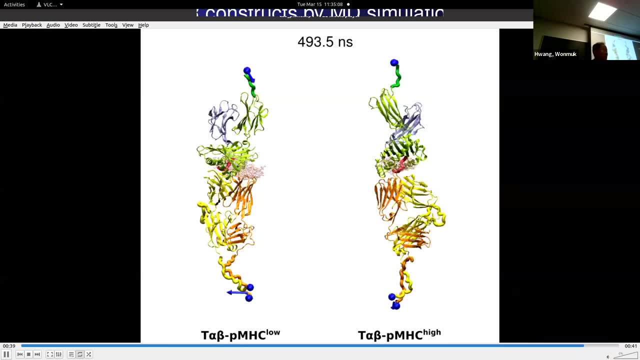 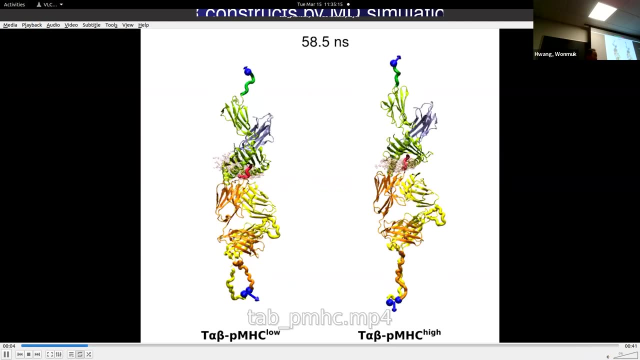 complexes. usually what people do is just apply high force, called the steered molecular dynamics, to, yeah, lead to dissociation of the complex within, say, 100 nanoseconds or something. uh, but if you apply very high load then you unbinding pathway will be different from the natural. 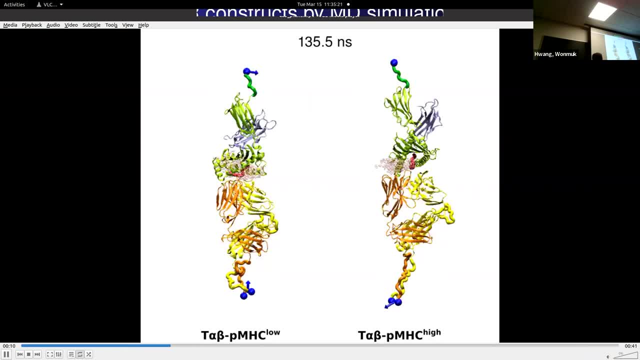 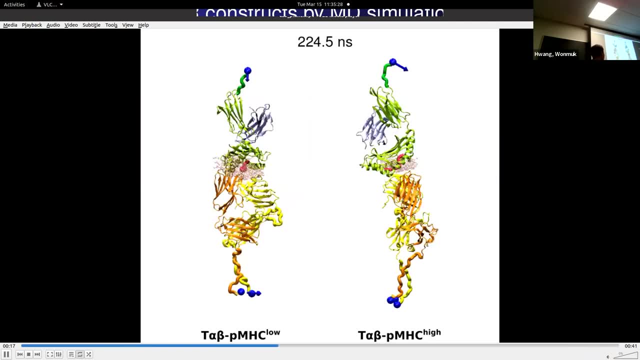 so what i uh was trying to do was to apply force and see how they respond. they can be done within 500 nanoseconds, because if you consider a propagation of sounds which is basically formed from here to there, it takes about 10 to 20 nanoseconds, so 500 nanoseconds. 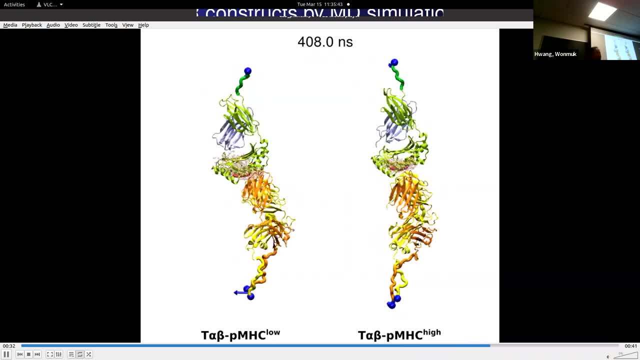 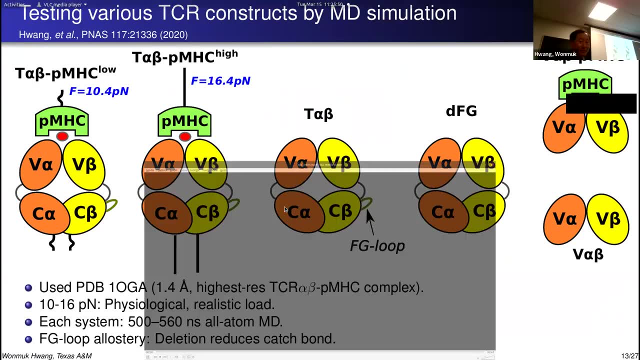 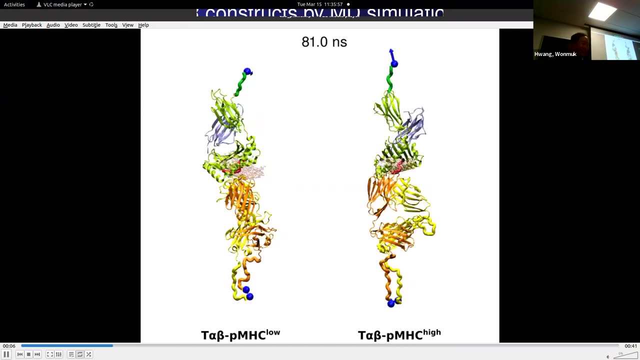 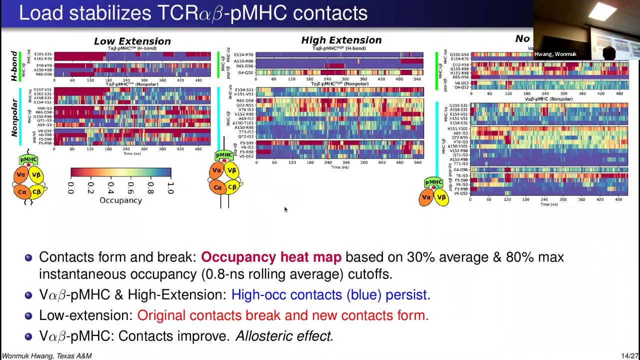 was long enough to see a confirmation of, say, equilibrium. okay, good question. yeah, so how do i see that the the bond is strengthening? here is the structural reorganization. it's not obvious what. it is right, so that'll come, okay, yeah, yeah, so i measured many things. so first, 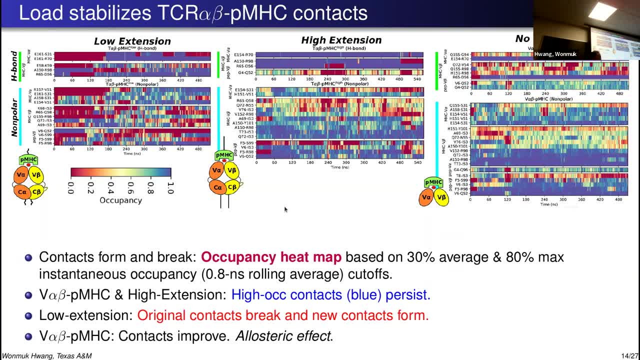 thing was the occupancy heat map. so you have the crystal structure. there are amino acid contexts of. if you run the simulation, this context form and break during the simulation. so i measure the instantaneous occupancy with this rolling average and actually plot it is occupancy in that with a. 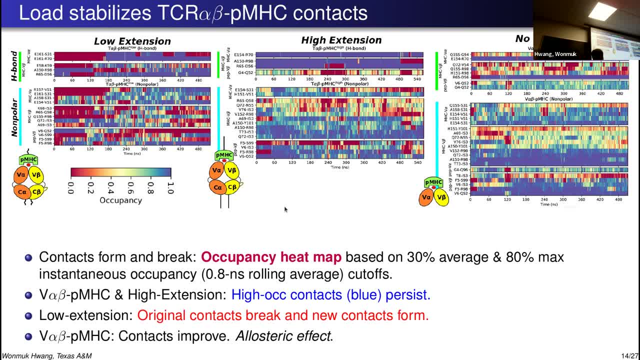 different or like occupancy cut-ups. so this is a reflex, a particular set of cut-ups. so what you can see is the low extension. there are many reds meaning that there are low occupancy. high expansion extension. there are more blues meaning that they contact more strong at high extension. 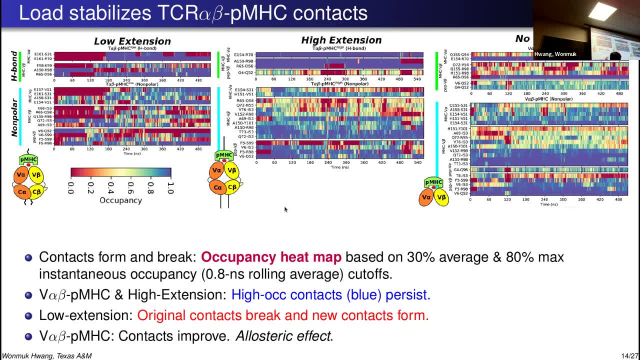 and no c domain. yeah, if you delete this lower part, actually the context increase, which means there is some allosteric effect from here to this domain too, yeah. so yeah, i measured like the hemming distance from the beginning and change this up a little bit, and i did a lot of analysis so i 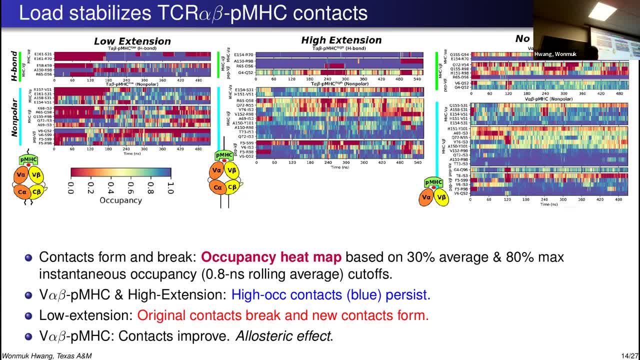 think this is the same for the general occupancy. and so, like i mean, i analyze the distribution, i mean spatial distribution, of this context within the interface, and all of them point that high extension or high load is better than low extension. yeah, i mean, you cannot calculate a. 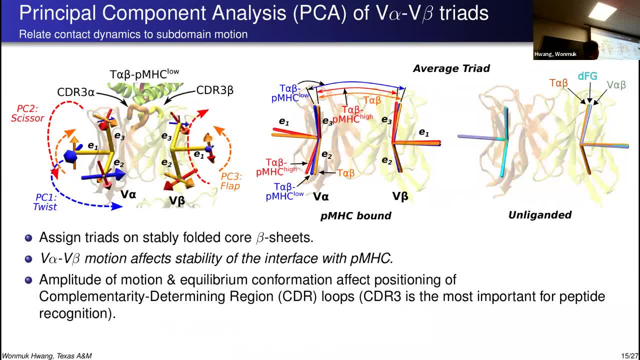 binding free energy, i mean with this method. but you can tell which one is stronger or less strong, and this is the confirmation of motion. that's the key. so i did this- uh, principal component analysis, using machine learning, i guess, and what's shown are the first three modes which i call. 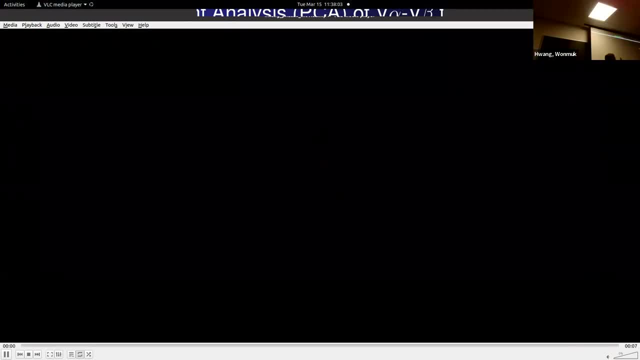 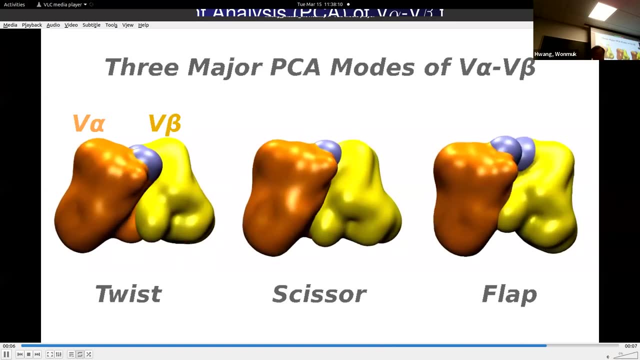 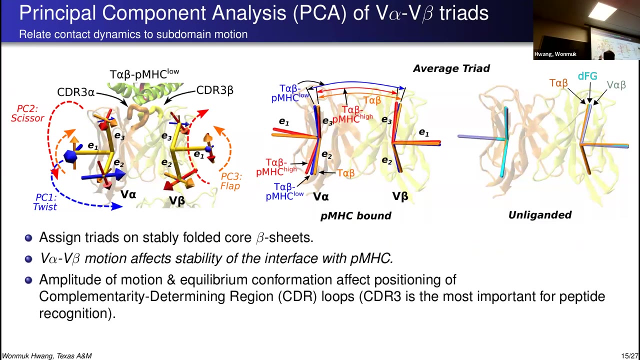 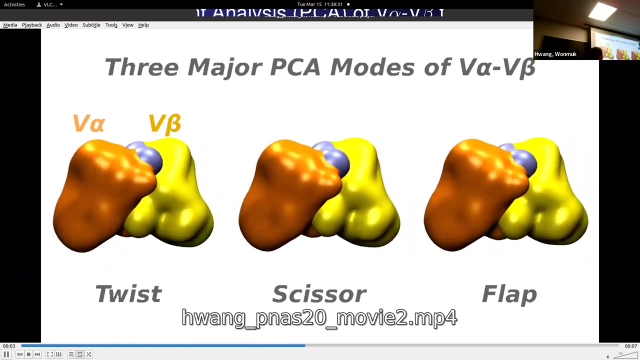 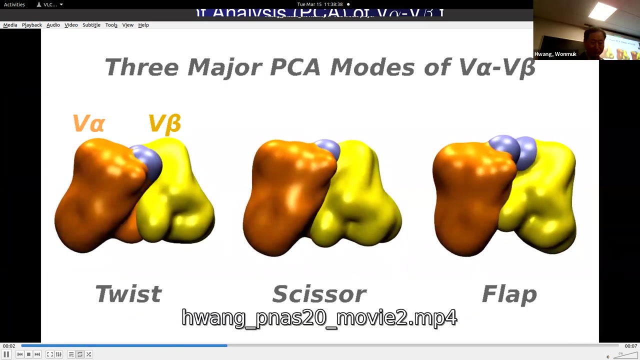 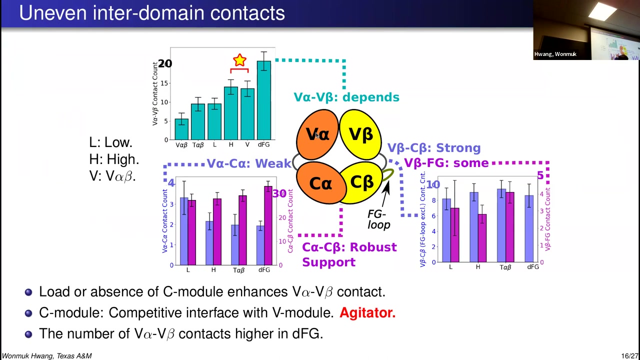 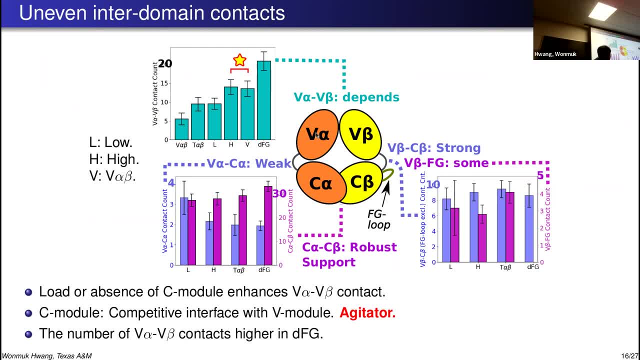 beta, and also actually look and found: oh there, the context are not like evenly distributed. first of all, between these two that we saw the motion, the number of contexts differ the most, depending on the system that you're studying, and between c alpha and c beta, the contact count is 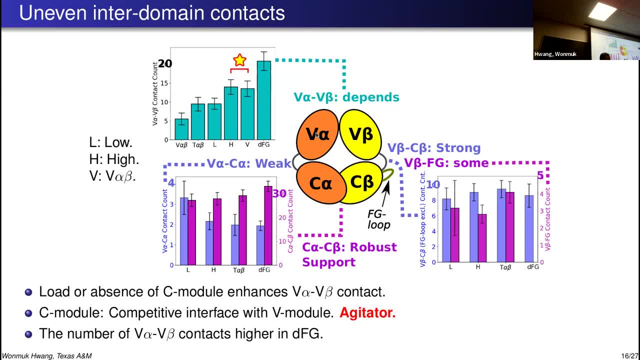 like a 30 or so. so this is the most robust based and between b- alpha and c- alpha. yeah, contacts only got up to like four, so these are weak, strong and there are some contacts depending on, yeah, the simulation condition and so on. so the main thing is: 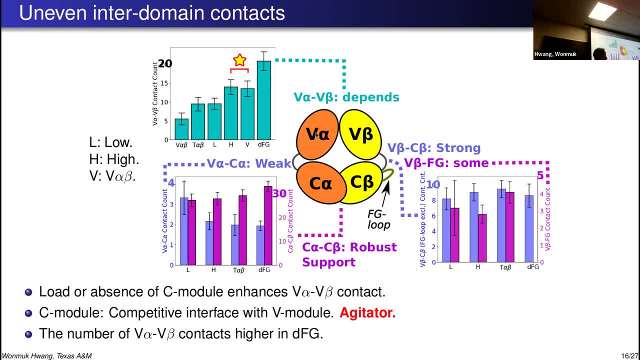 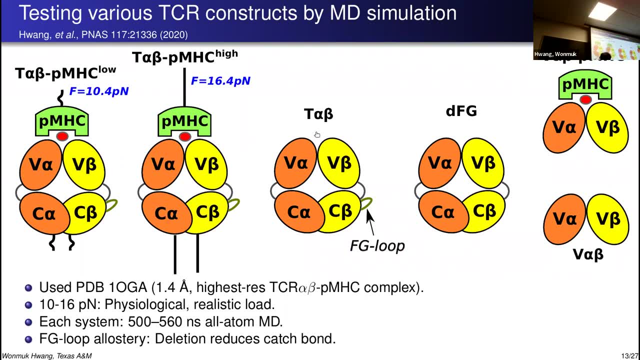 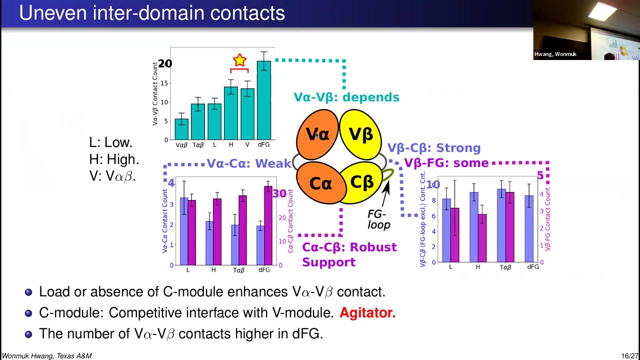 the distribution of contacts are uneven and when we go to that picture in this case you need to satisfy three: body contact, which is not trivial, so if there is a domain motion here, you can actually control how well they fit. yeah, so that's the idea and the c module is an agitator actually. 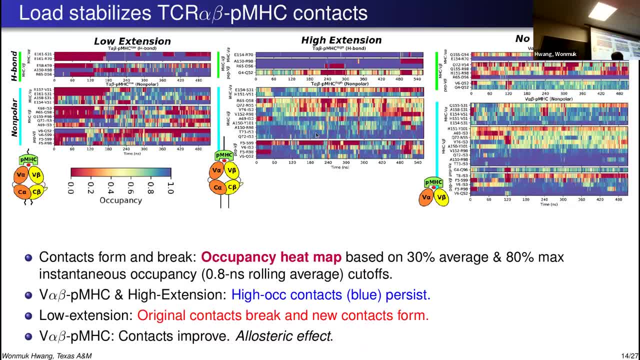 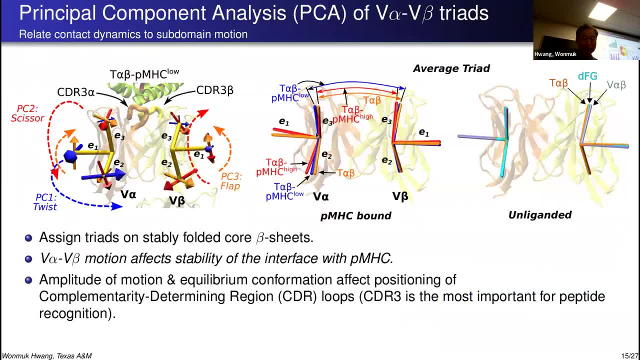 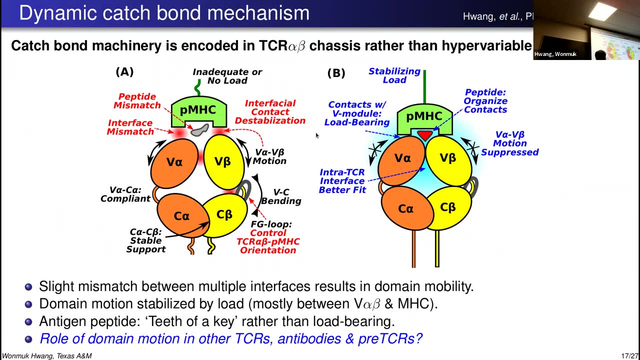 because without the c you can get better contacts. so the c module was there from evolution or whatever to destabilize interface without force. so, skipping all the other analysis, here is the lesson i found. so without the load these domains are not like perfectly fit. it's topologically closed structure, so 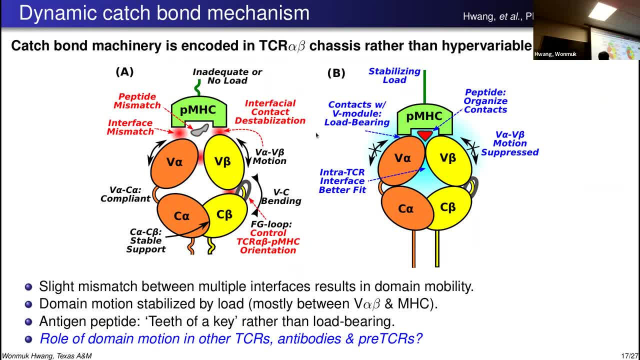 you cannot just deform them and just easily, yeah, fit them. and also, if there's a mismatch in that type, the same thing happens. and when there's a load, then the there are these contacts between the mhc to these b domains, to pull them, to sublize their contacts. 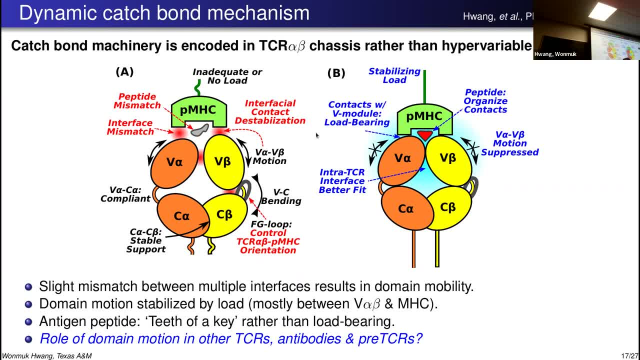 so these domains don't move, then if the peptide is the right fit, then you can maintain the interface. so here, yeah, the mismatch seems to be there from the like basic design of this, that is a receptor, and the catch bond is achieved by stabilizing this domain. 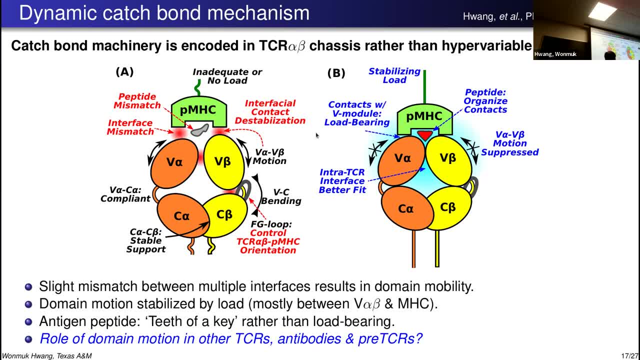 and before this work, people thought the right peptide will be the load bearing, but actually it's not. i mean there are only a couple of contacts between the peptide and this, whereas there are much more here. so peptide is more like is a teeth of a key that filters the right fit, but once the 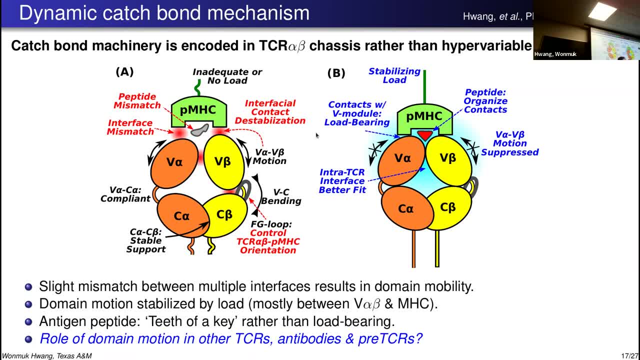 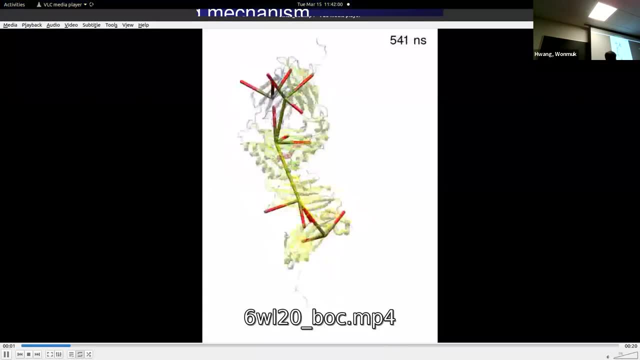 fit is good and the load bearing contacts are different. so currently what we are doing is we study this for our different types of t-cell receptors and the pre-teaser receptor. this is a simulation of the pre-tcr and, yeah, i use the basically the same method. 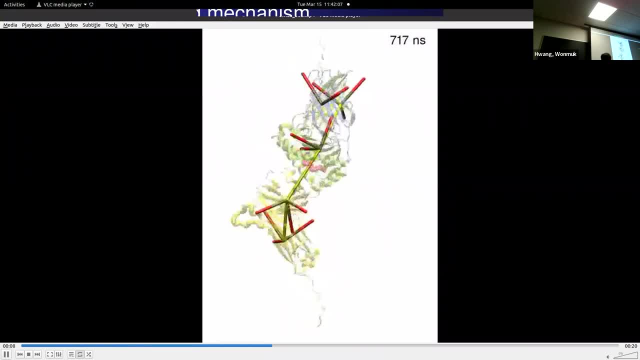 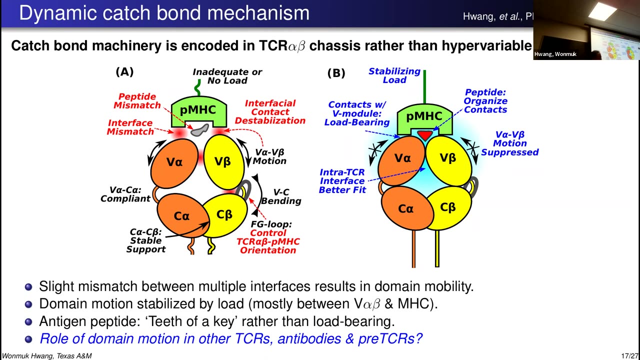 that i use for the dna to study the relative motion between this and that, that and and so on and so forth. and i mean, if you think about making receptors as, uh, sensitive as this, you can make this as like a one-shot. you know so, actually, when t-cell 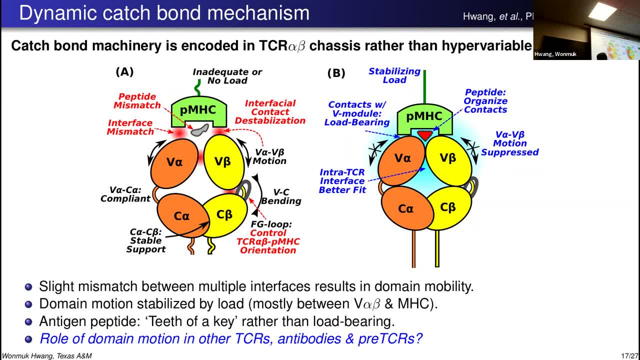 receptors develop. uh. this beta chain is first expressed without the upper chain and their contacts are of course like screened. then, after a certain group of contacts are selected, then alpha chain is expressed to finally get the mature tco. so the problem here is okay when you don't have the upper chain. 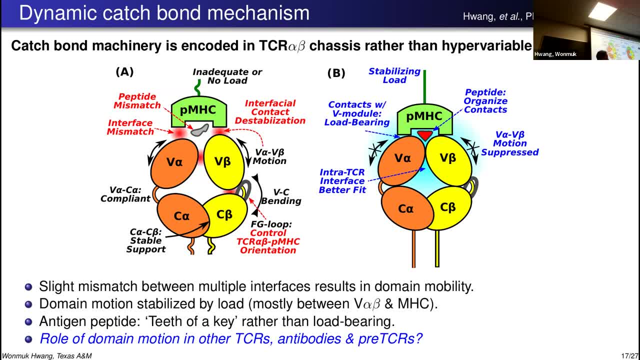 the contact between this beta and pmhc is not going to be used in the end. it's going to be only a transient contact. then what do you mean by the right or wrong contact here? so those are the questions that need to be addressed when there are experiments. 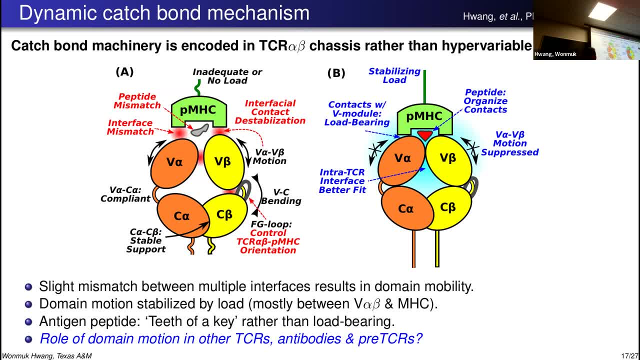 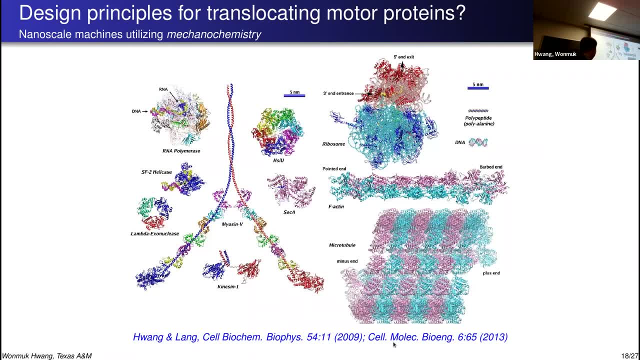 but the atomic picture, i guess, can only be obtained from uh simulation. yeah, so i'll be quick in the time here. oh, time is good. yeah, move to the motor protein. and yeah, i was fascinated with this motor world, and this was from a regular paper i wrote. 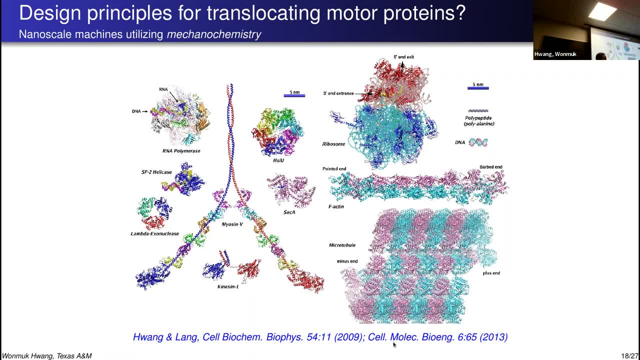 with a metal, and the main output of this review paper is this picture actually, yeah, five nanometers can be obtained from a nanometer scale box, so they are actually the same scale. so these are the motors: rna polymerase and ribosome and the other dna modifying enzymes. 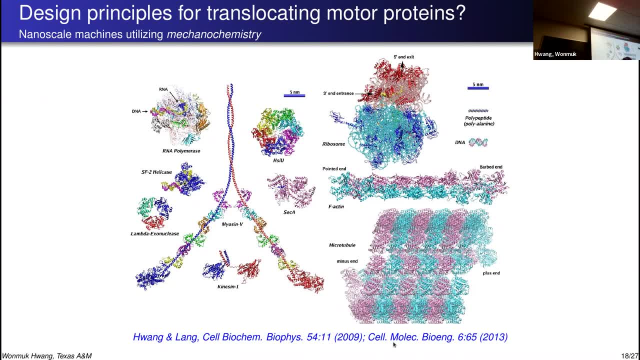 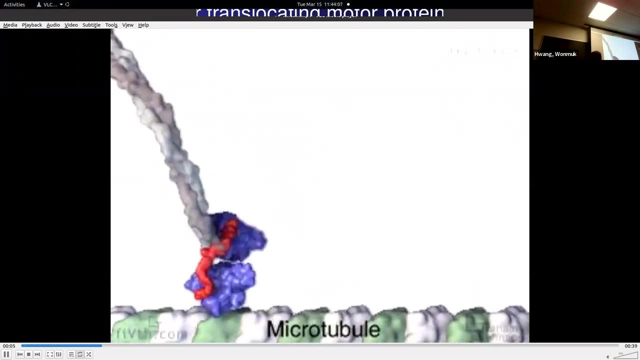 myosin 5 and kinesin, and these are the tracks where these motors walk on. and yeah, the understanding develops from the experiment first. so this is made by ron bale's group at uc san francisco, and laro with his imagination some. 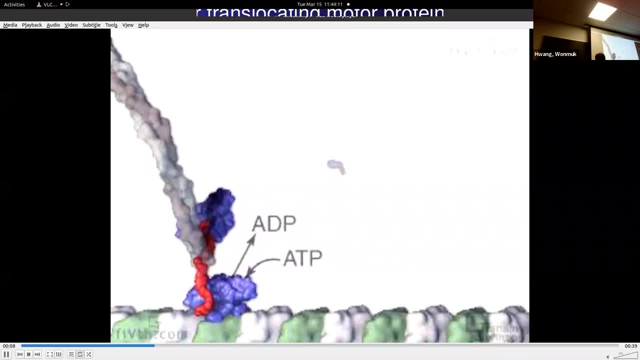 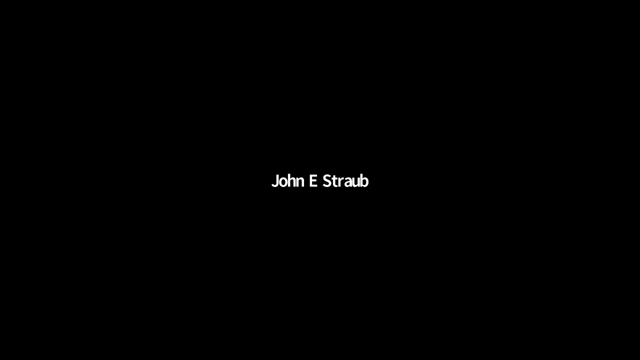 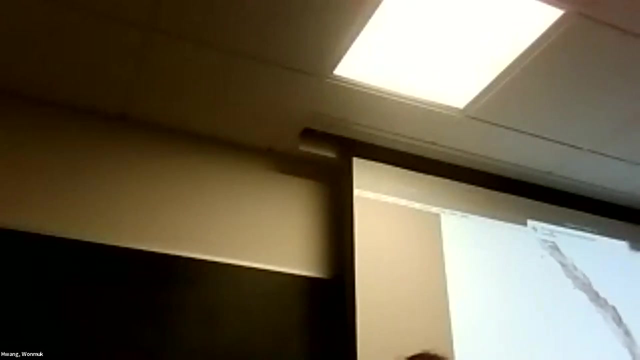 of the experiments that were conducted in this project were mostly based on the information collected by the laboratory, and the information collected by the laboratory was actually a very, very, very extensive research that was done in the i very, very well so. so So there are kinesins that walk backwards, so they actually switch this domain between 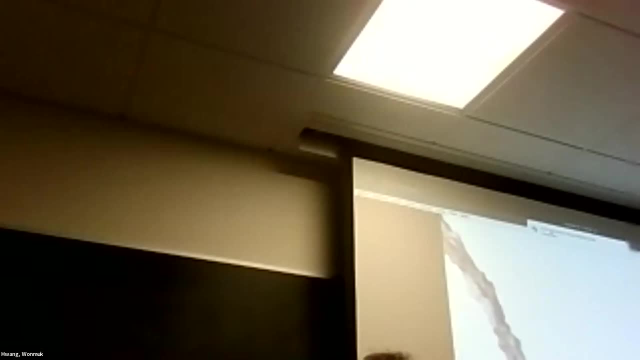 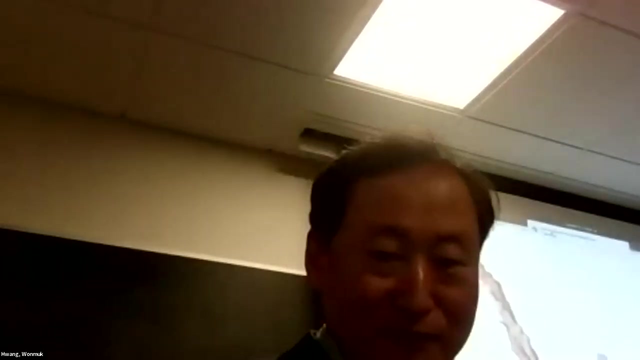 the two kinesins. they actually switch the direction out, although the motility is quite impaired if you just switch this. So yeah, it's not like a point object. that does what I mean. we have to understand basically the atomic details here. 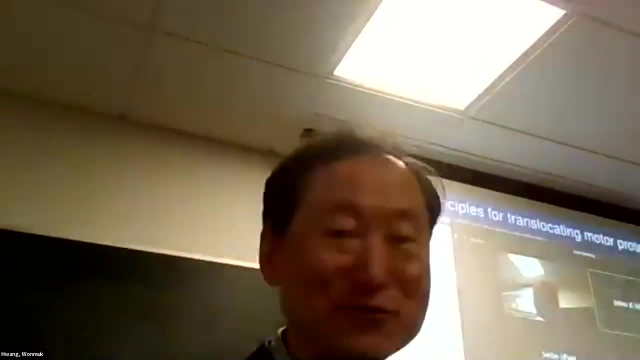 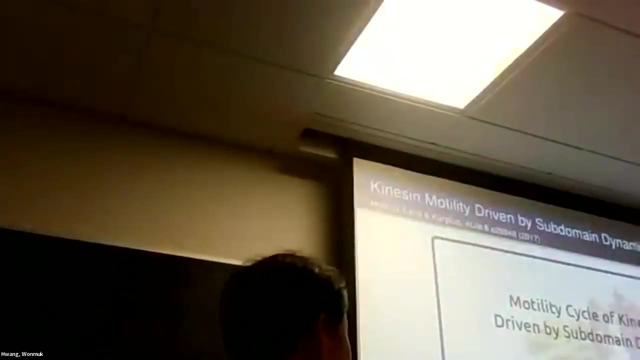 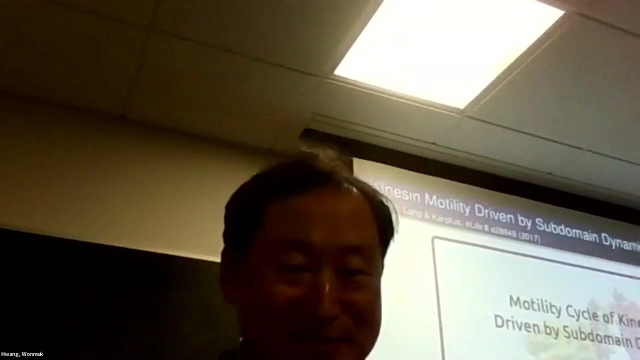 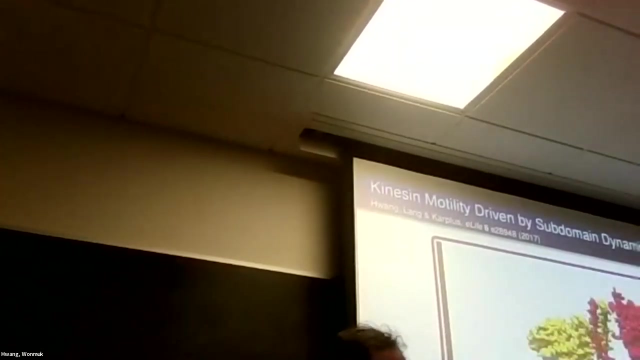 So I did a bit of simulation, using Antone actually. and yeah, without explaining what the simulation was here, this is a supplementary movie explaining the concept developed. So it's less imaginary, but still a lot of it is imaginary but a lot of it is based. 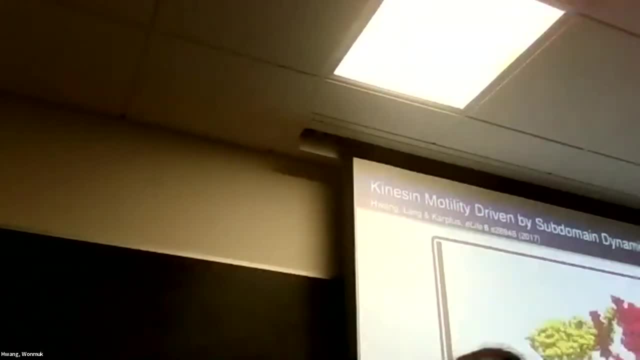 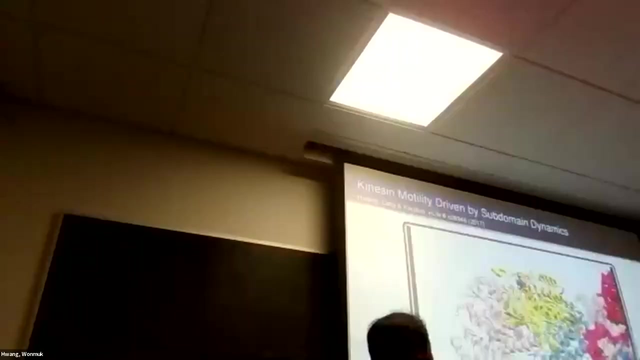 on simulation. So yeah, the front head explores the binding site by kind of diffusive search and the rear head it has a bound ATP and note that they have to make steps. so the interface has to be marginally stable. 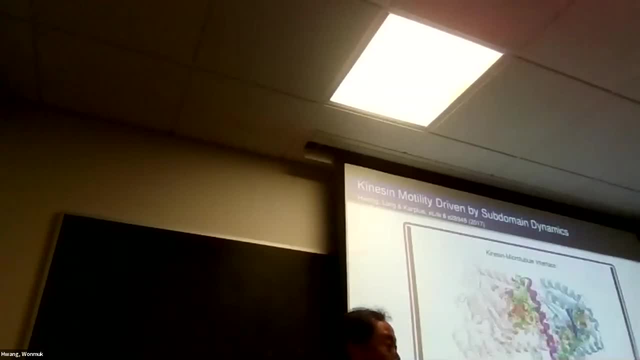 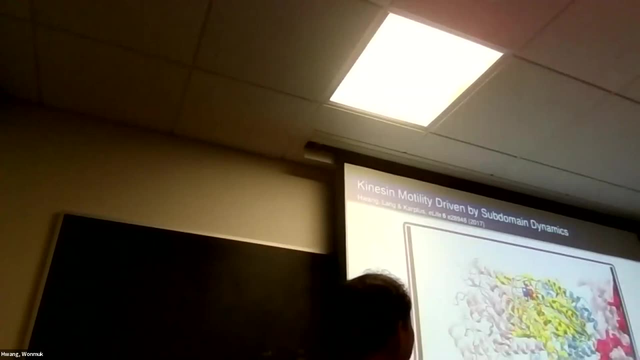 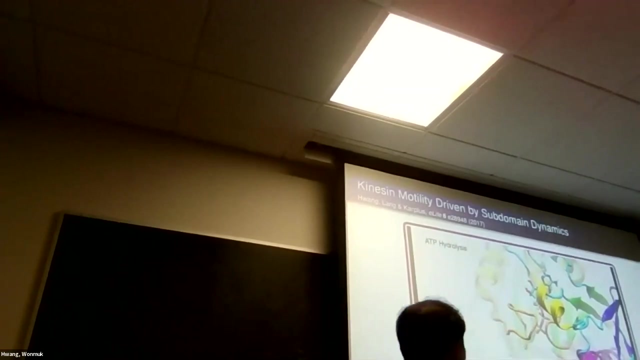 Actually there are water molecules going in, Okay, So it's a wet fit, Yeah. Then we pay attention to the ATP and these are the switch domains, and the simulation shows that these switch domains are not just rigid, they actually move quite a bit. but 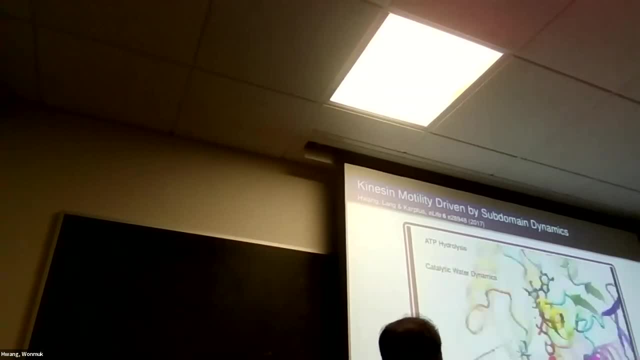 they still move within the density of electron, density of cryo-EM maps. So there are these mobile switch domains and the conformation of ATP in the free state and the bio-state. this is more based on the crystal structure. There is a torsion developed. when the torsion doesn't break the bond, but I think it'll. 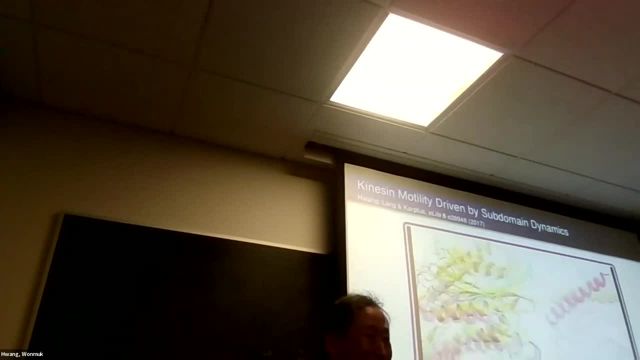 help with the attack by water. Chang may have more to say about this. Yeah, anyway, so ATP hydrolysis make this weaker, bound, which we don't know exactly. Okay, Okay, Okay. So the ATP release in the front. in the simulation you can see the ATP pulled out. 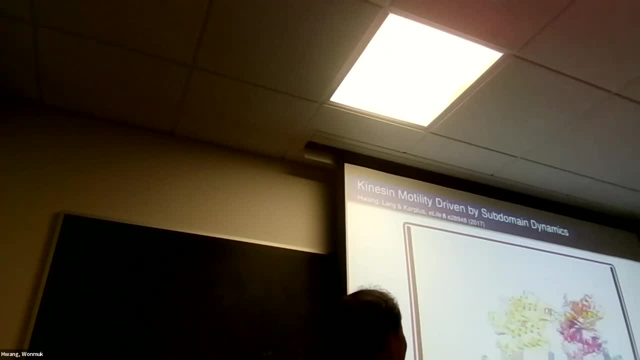 but from here to there is just a visual demonstration. Yeah, now apostate nonuclear type, and then this releases a PI that was seen by simulation and obtain is helped by this moving loop. The loop is pulling out the phosphate, So in the ADP state. 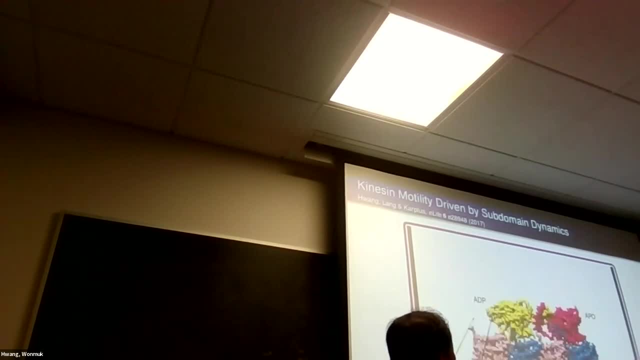 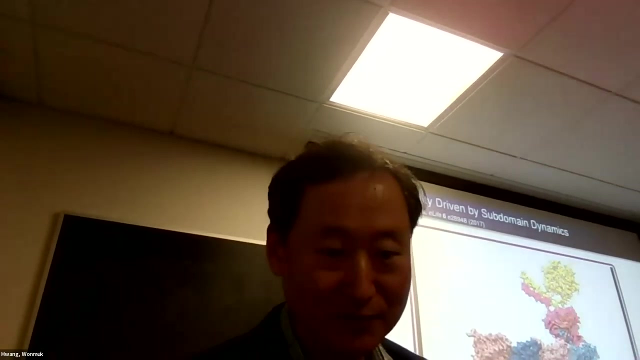 the binding becomes weaker, then this can detach. So this has kind of moves around which is not well understood right now. Did you just make sure that you're still sharing your speech? I don't think so. Okay, let's see. 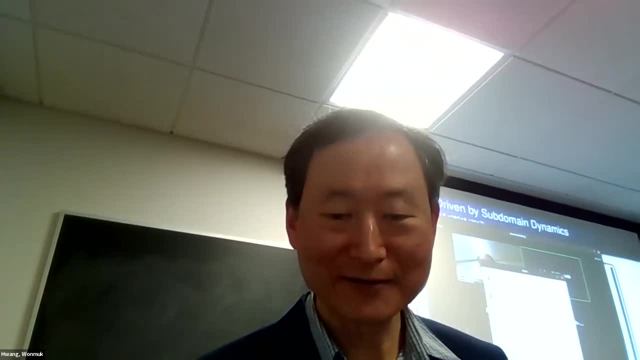 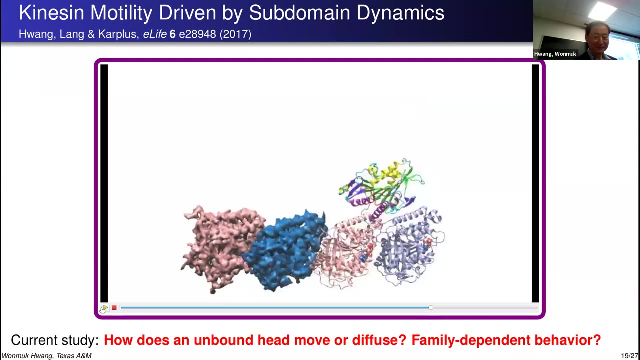 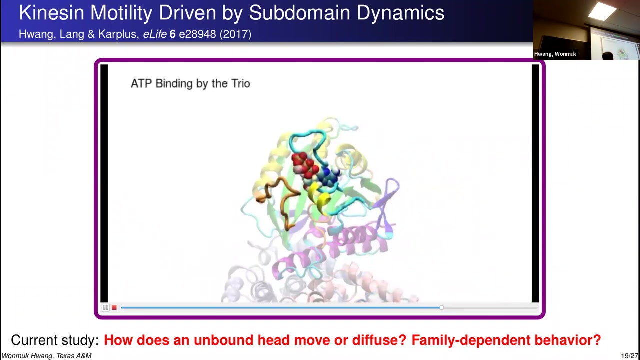 I'm not sure. Oh, sorry, Now you are. Yeah, thank you, Sorry. Yeah, then in the front end, there is ATP binding going on and the thing is ATP, this is adenine part, which is like hydrophobic part. This is the phosphate. 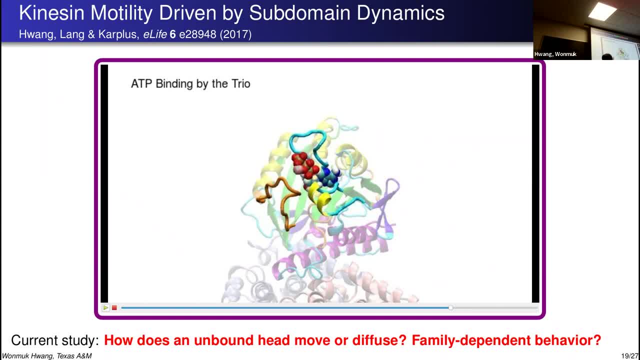 triphosphate, which is highly charged than hydrophilic. So if you just put this near kinesin, this part wants to go in. So there is an electrostatic guidance for this negatively charged part and also what we will see is that these moves. 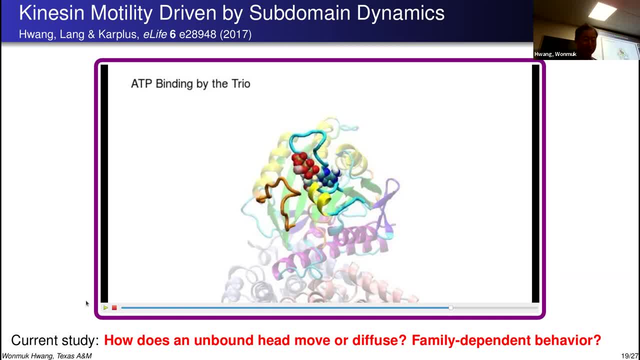 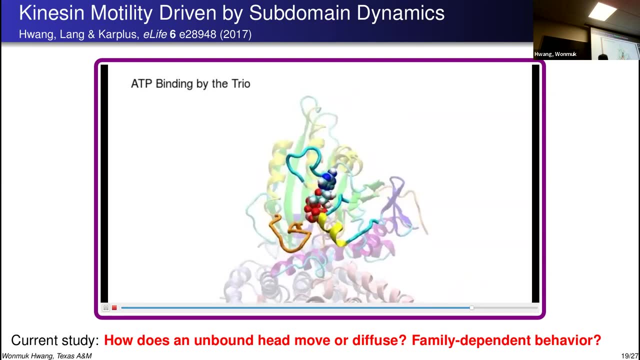 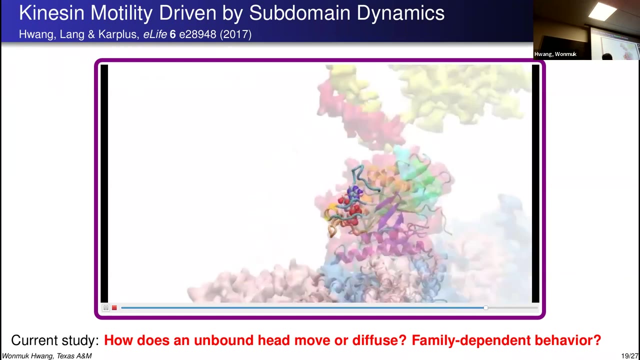 these mobile domains actually help with their orientation and binding. Yeah, this is the actual simulation that they are basically caused by these three. and yeah, the binding is. I just made it happen. Yeah, so ATP binds to the front end. then we have that negligor dimension, and how does that move? 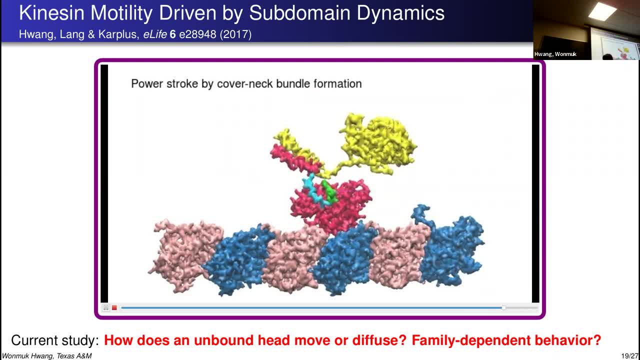 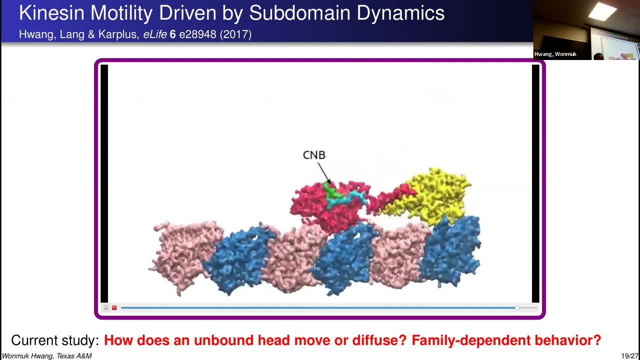 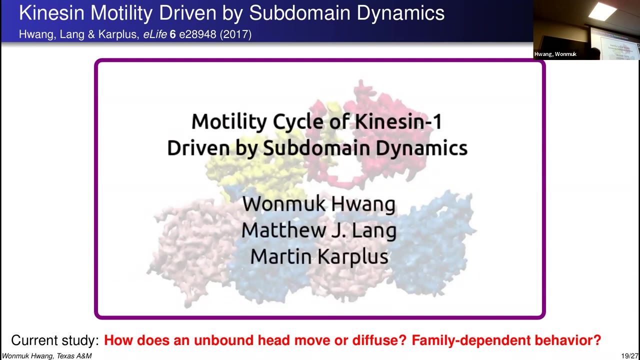 There is a small N-terminal strand called cover strand, and they form a beta sheet and the beta sheet has a forward bias to push this forward. So this is how one step is done in kinesin. So yeah, there are other questions about this- conformational change and so on- but what's missing? 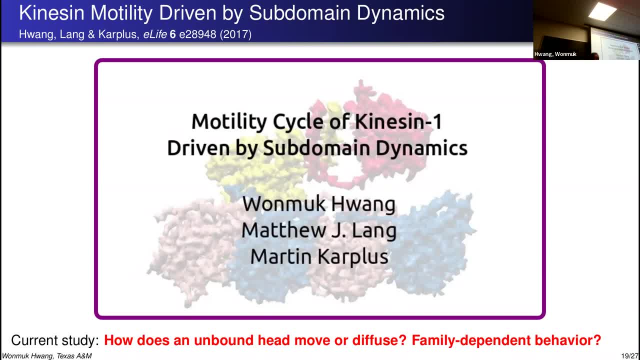 here is how they move. when they are moving, Yeah, like unbound, or how do they diffuse? In those questions, I guess, the least understood so, which is what I'm studying right now, and those questions also relate to the family dependent. 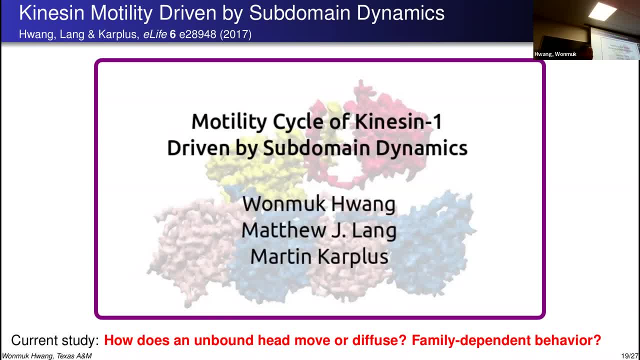 behavior. Yeah, the simulations do not have a load on them. There's no load here. Yeah, Presumably the load has a huge effect. right, It should drag along a very large time. Oh yeah, Yeah, Is it the load-free case? What sort of load would you need to pull it backwards, right? 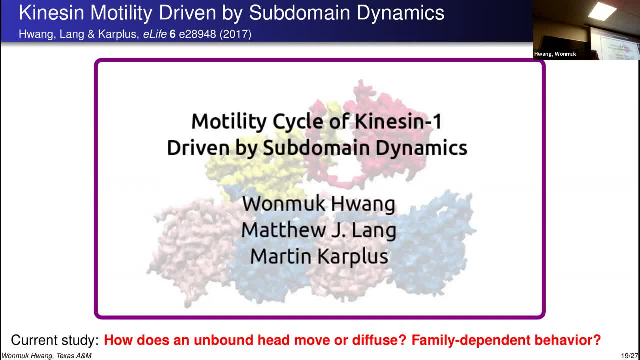 Oh yeah, So the load has to be more than, say, 10 piconewtons and so on to stop. I mean, kinesin is towards at seven piconewtons, So if you apply seven piconewtons they cannot walk anymore. 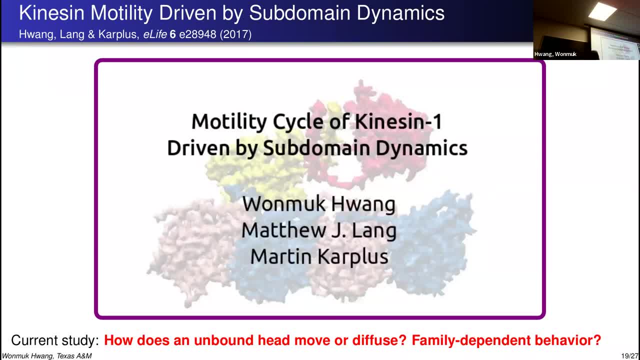 Yeah, and the most low-sensitive phase of this cycle is when they try to make the poor step. Yeah, if you pull back, Yeah, what I showed was when they form the beta sheet, then they can resend the load and move forward. 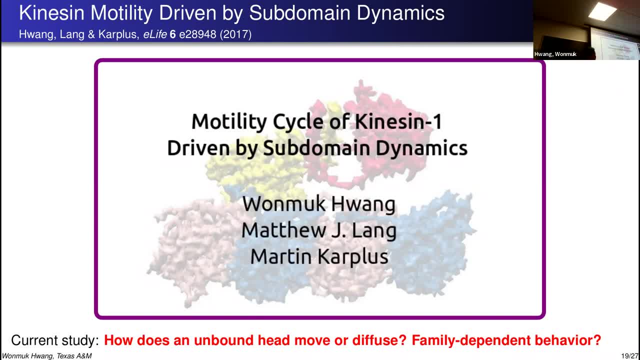 If it's a single strand, I mean, there's no way they can send the load, yeah, Yeah. and there are other kinetics that do amazing behaviors, like they diffuse and they depolymerize microtubule, And yeah, they stabilize microtubule, and so on and so forth. 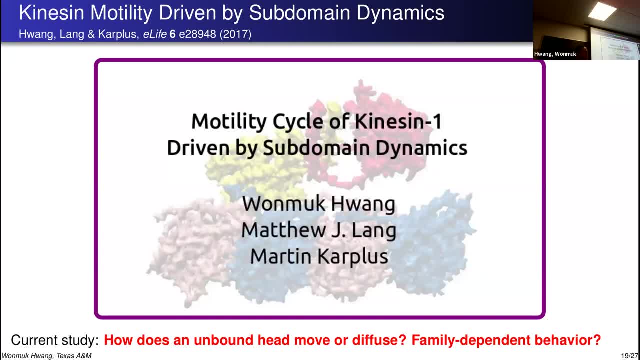 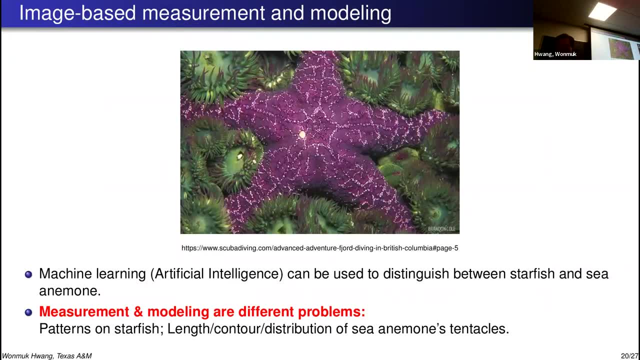 So there are quite a few questions left in the kinetics family still. So so each hour here, for the remainder like a few minutes. So this is like a offshoot of my biomolecular simulation. The question is: yeah, if you see an image like this. 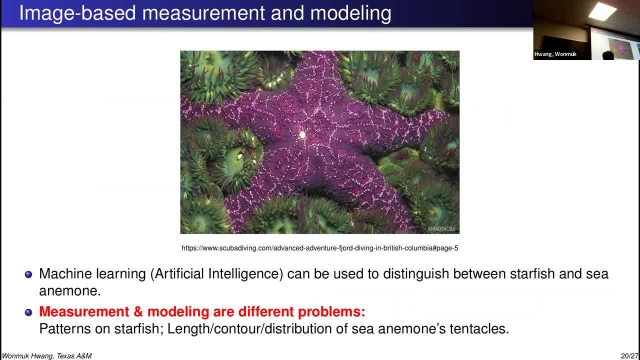 you train them through some machine learning, then you can tell: this is the starfish and these are sea anemones. But if you want to study their patterns or like less distribution or motion of these tentacles, that's a different story And people have studied or generated this. 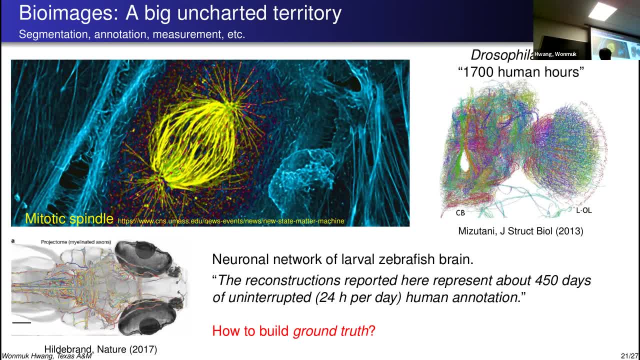 models of different structures. Here's a mitotic spindle- I mean, this is an experimental image- and this is a drosophila braid, a neuronal network, And this is, I think, a zebrafish larva braid. 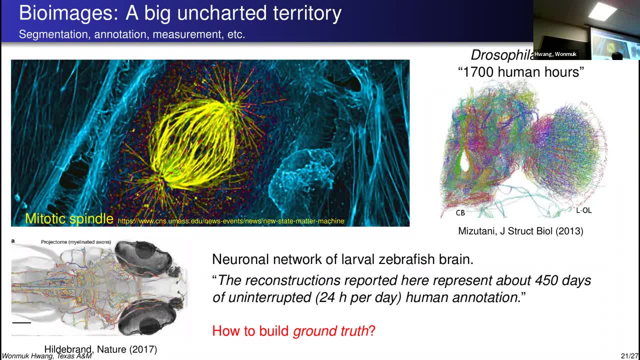 So there are this traces And, if you want to do supplementary information, they bought how much effort they spent like 450 days of uninterrupted of human annotation. So yeah, with all this development of machine learning methods and so on, they there are tools that assist with this tracing. 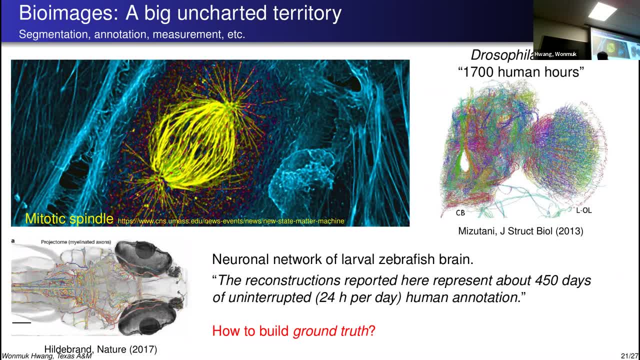 for this in the end of like businessman And the problem is okay. So suppose you did it for one one system. can you serve as a ground truth? the connectivity is all different, so here the ground truth is, yeah, out of question almost, and i mean i got into this, uh, based on my earlier work. 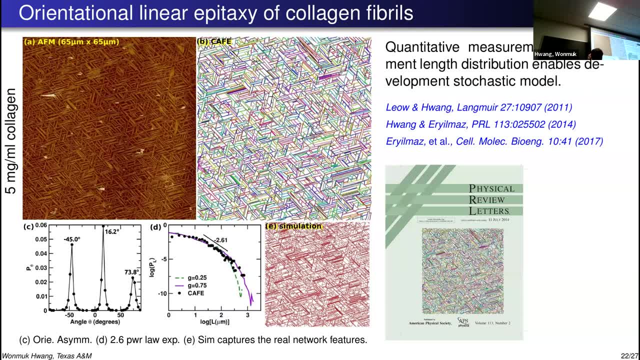 so we studied this uh collagen network on mica surface in like afm image so i was developing like theory about their natural formation, then wanted to measure their length and it wasn't easy and actually it happened in the end. so they, these elements, are colored differently, meaning that they are registered in the program individually so i can measure. 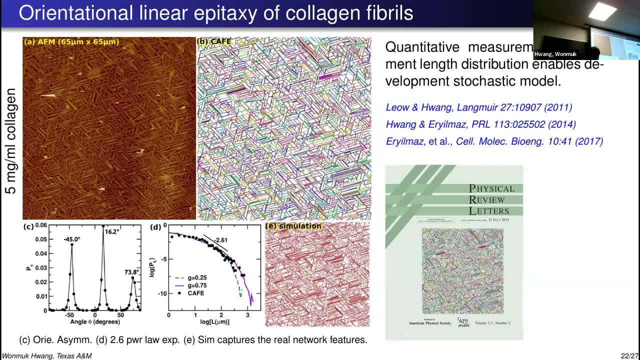 the orientation distribution so you can see, uh, two peaks minus 45 and 16.2 that are major and 73.2 is oh, this, so you can like roughly feel there are less filaments in this direction than that or those. yeah, you can measure this, uh orientation distribution and you can measure the length. 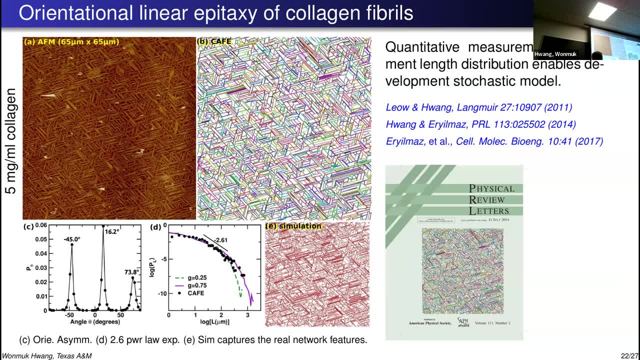 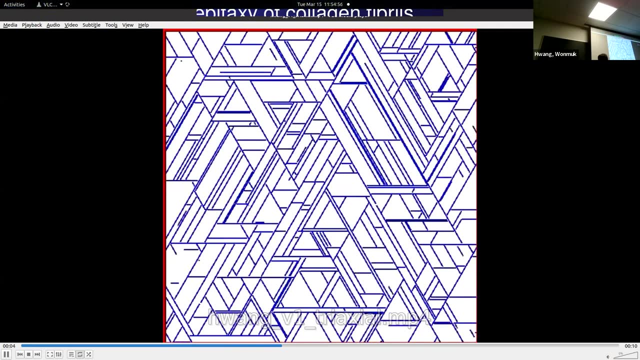 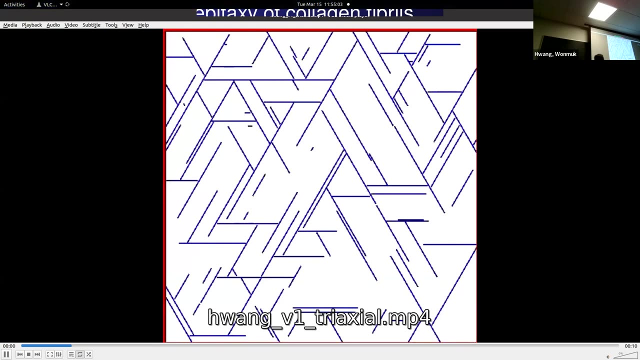 distribution in the low block of scale and there is a little bit of power- low 2.6- showing that this is like a fractal structure. then you can build a stochastic model of this structure formation. you start from like empty space, then you create certain uh filaments at certain rate and you grow them in certain growth. 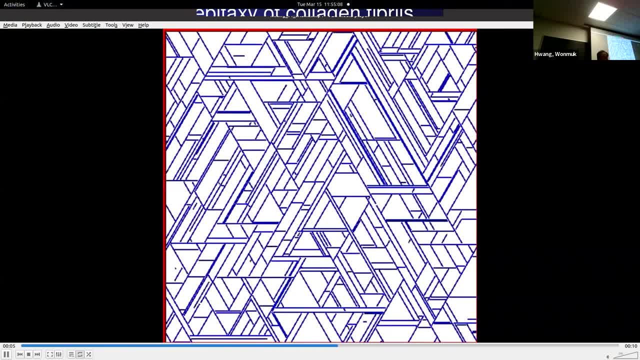 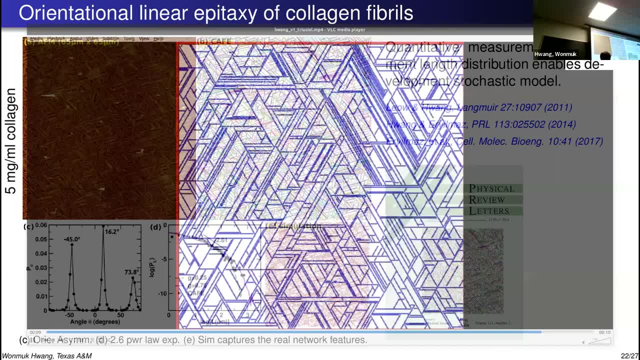 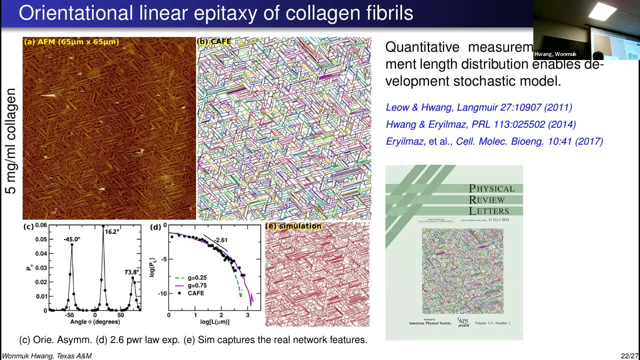 rate and growth stops when they hit other flags like great screensaver. yeah, okay, yeah. so this is the simulation and the nice thing is that you have this experimental uh data. then you vary your like growth rate and see what is the differential risk growth rate that can match this distribution. so once you find this growth rate, then you can do the simulation. 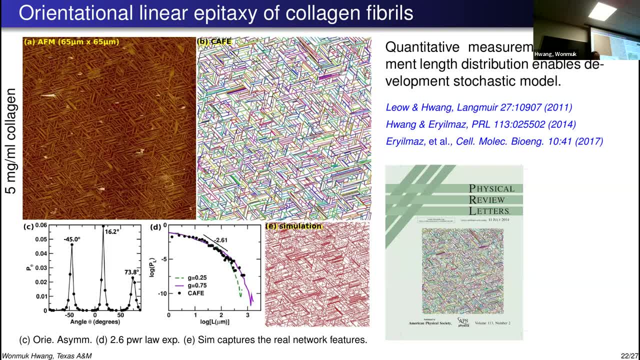 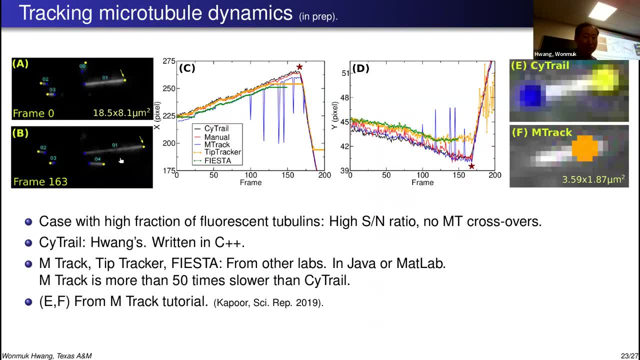 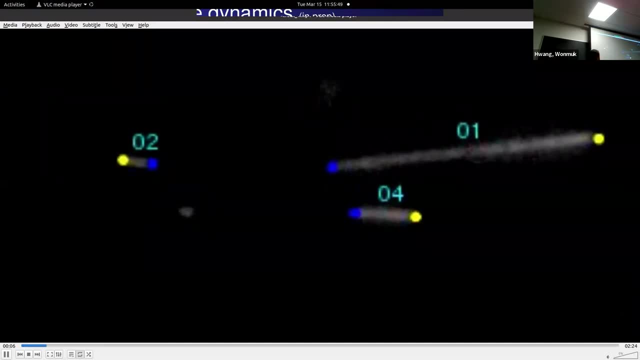 and it qualitatively matches the experimental officer. yeah, so this method is further developed. and now, uh, i'm doing this, uh, microtubule tracking. so these are the microtubules on, uh, like two dimensional substrates. so there is a uneven growth. this is a fast growing it. 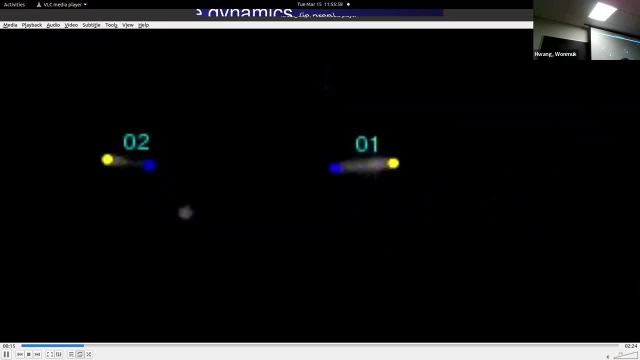 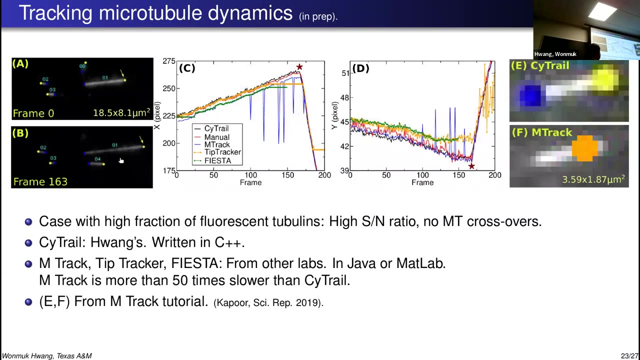 and they do something called uh catastrophe, then they polymerize it. so this needs to be tracked to get their velocity distribution itself or how frequently they do catastrophe, and here when the efforts have been there previously. so side trail is the uh yeah program that i developed which actually traces the manual the closest and the most advanced. 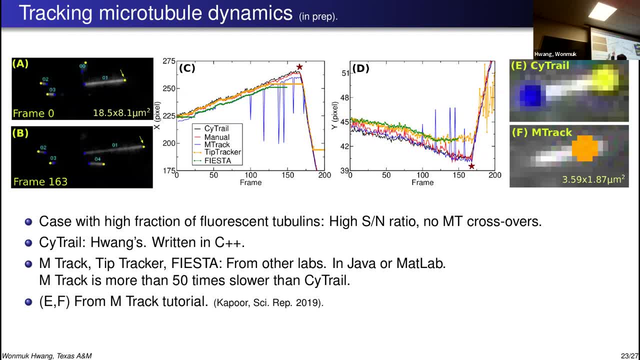 so far is the m track which you can see. there are occasional dropping and a little bit of lagging here, and so, just to be fair, i downloaded images from this mtrek website and applied their tutorial and applied my, and actually the ends are better tracked in my method. this is, yeah. the problem is these are 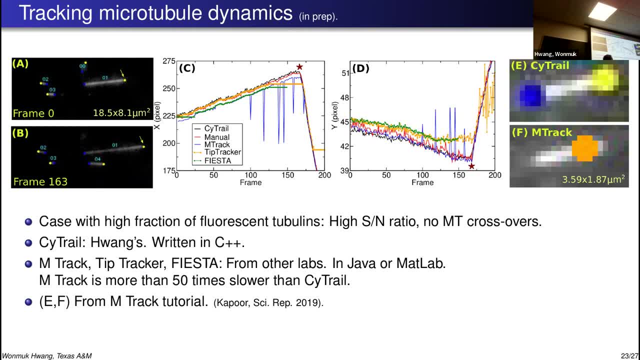 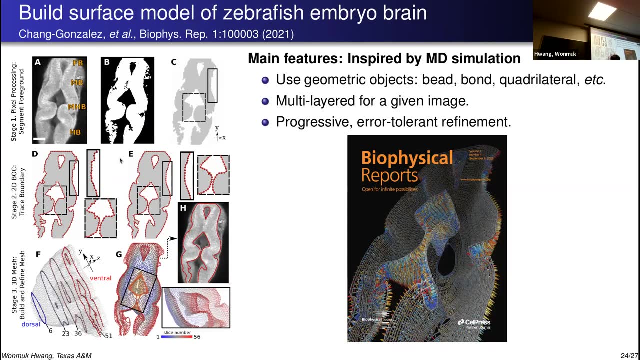 written in, uh yeah, matlab or java, so anybody can use these. right now. this is script based, so it's just difficult to use. yeah, but this has a lot of applications. i mean, yeah, although this seems to be very different from simulation, the ideas underneath took from our md simulation. like we 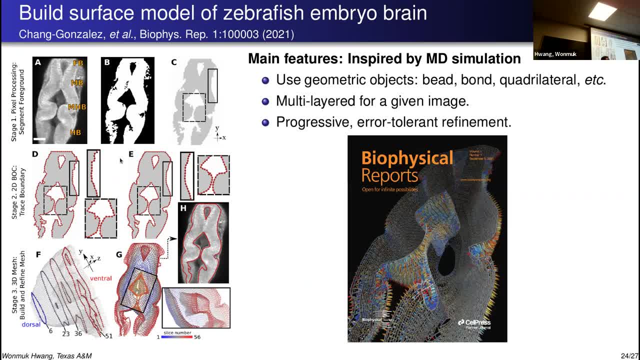 can use, uh, these and bonds and these quadrilaterals, the simple objects, and assign the objects to structures, and in this case is a zebra fish embryonic brain. so these are the neural epithelium. so if you just apply just simple binary thresholding, it becomes noisy because of 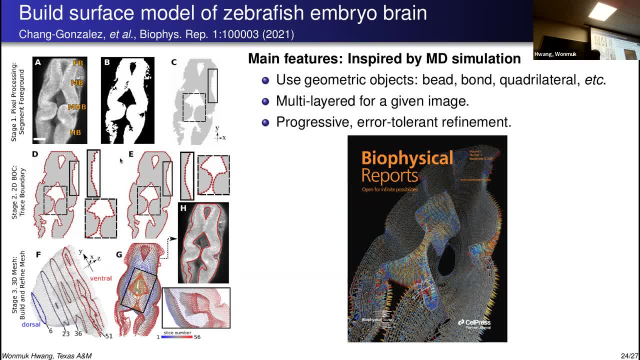 this background. but there are a series of refinement procedures- progressive and aeropower an image. we can separate them into different channels and look at different aspects. So the combination becomes this nice surface map with starting from quite noisy images. So actually this biophysical refers, or that was the first issue when we just covered the first issue. 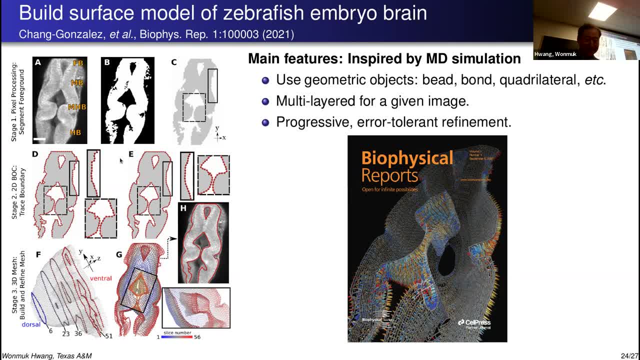 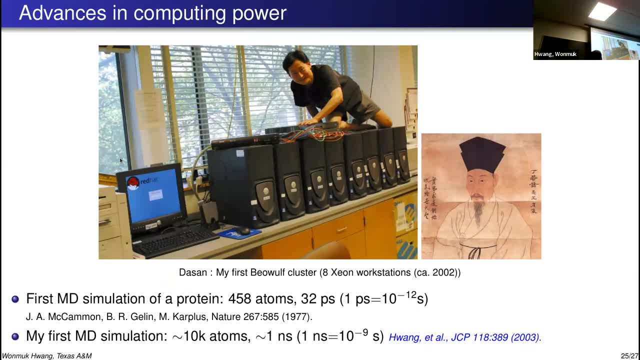 Yeah, so many interesting things going on. The yeah, yeah. the fun thing is that I like this programming and, yeah, debugging and so on. So this was- yeah, it's already 10 years ago- my first build cluster that I built, So it was quite exciting. So this was a shot And yeah. 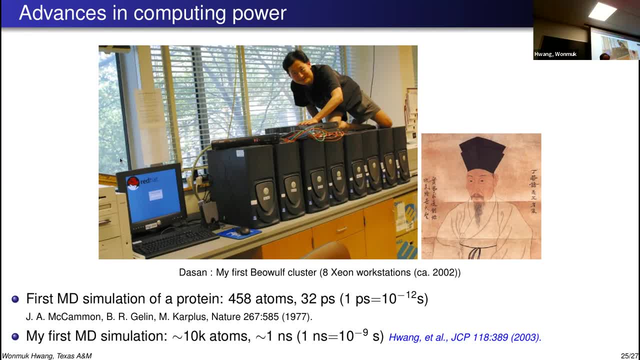 I won't mention why this doesn't come from this Korean scholar's name, But yeah. So the first simulation was from Martin Koper's 32 picoseconds, 450 minutes, And with this cluster I was able to simulate 10k atoms about one nanosecond length. And now 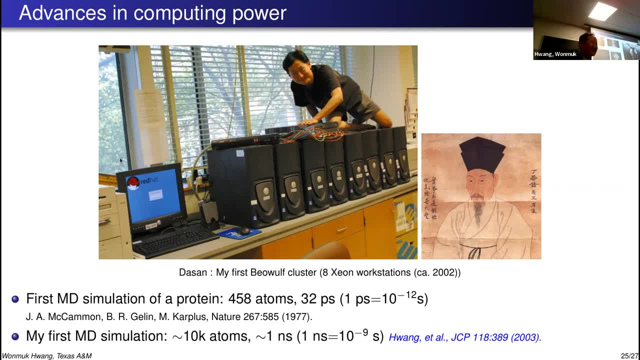 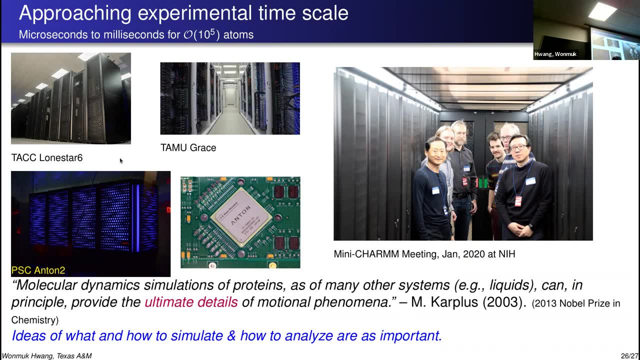 the time for building your own cluster is almost gone. We use all this larger scale. And yeah, there's that. Yeah, we took the filter, Yeah, Anyway. so yeah, Martin mentioned: yeah, MD simulation can see the ultimate details of motion of phenomena. That was quite 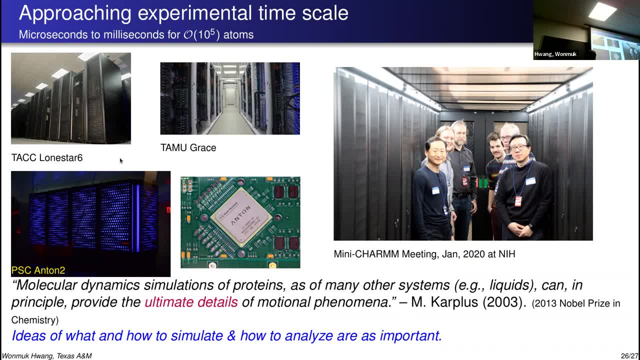 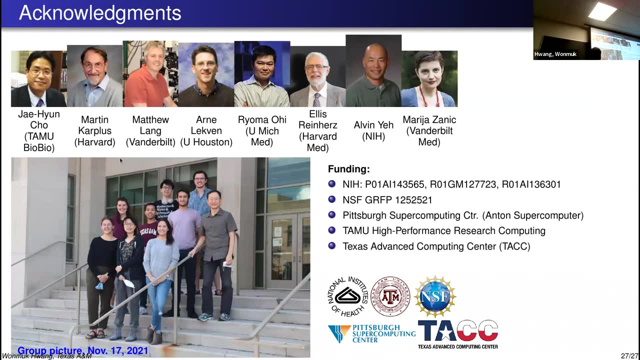 right statement, I think, But I think you have to do know what you are simulating and how to analyze and so on. So these all are have been, yeah, great and exciting developments so far, And I'd like to thank many people, So I'm just like showing relatively recent people. 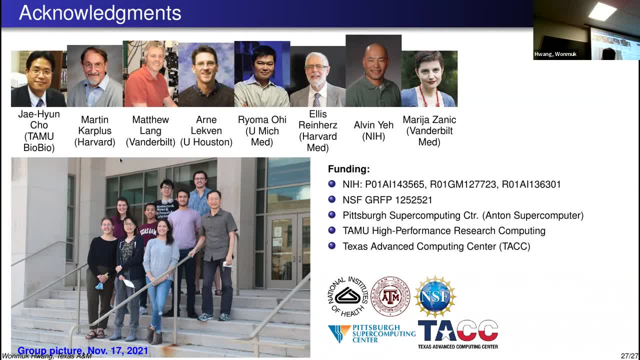 And the current active collaborators are Jay Henshaw, Martin Koper, Matt Lang, Alice Reinders, Maria Zayn and my group here And with all these funding sources and computing resources. And now I'd be happy to take questions. 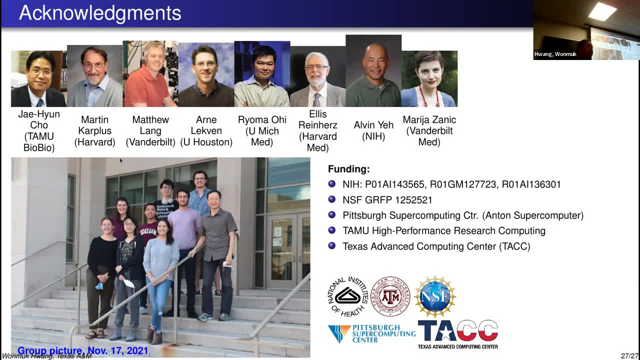 All right, It was really impressive. you know brands of things that we have. we have learned, So open for discussions. Yeah, Do you know what the capacity is to code? Oh yeah, that is GTP hydrolysis. So microtubule, I mean if it does polymerizes in one direction. 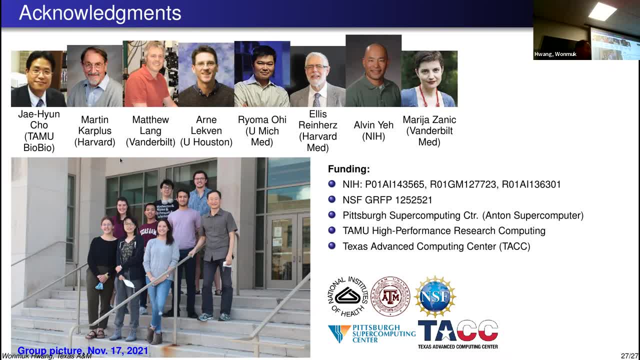 that means there must be free energy cost. So free energy is supplied by the GTP. So when a tubulin monomer has a GTP bound, it's prone to polymerization. So they polymerize. But as they age GTP hydrolyzes. So this G hydrolysis. 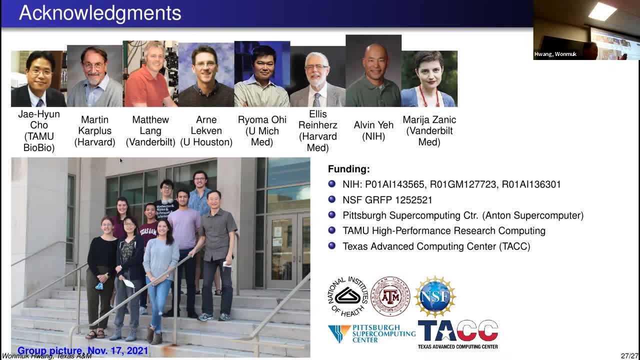 follows the front. So when it goes, reaches the front. if everything is like in the GDP, they, they, depolymerize, Yeah, so it's the balance between hydrolysis rate and the growth rate. Yeah, Yeah, I have a question about the first of all. thank you for talking. that was really. 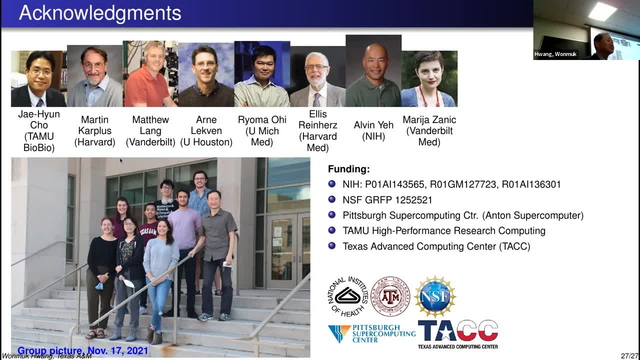 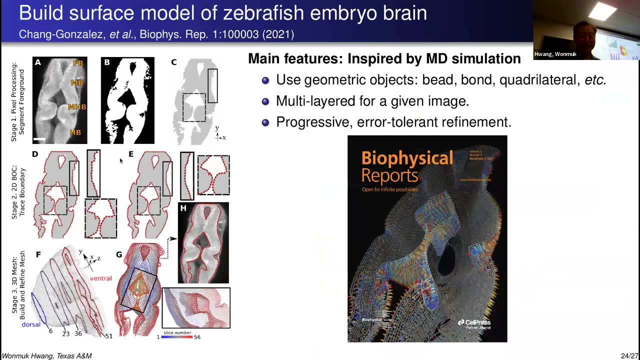 interesting Question about the bio, the recognition of the peptide in the immune systems. Did I understand correctly that the the weak binding that it's supposed to detect? like you mentioned that? it's very binding, Yeah, So that's the mechanism that's specifically built. 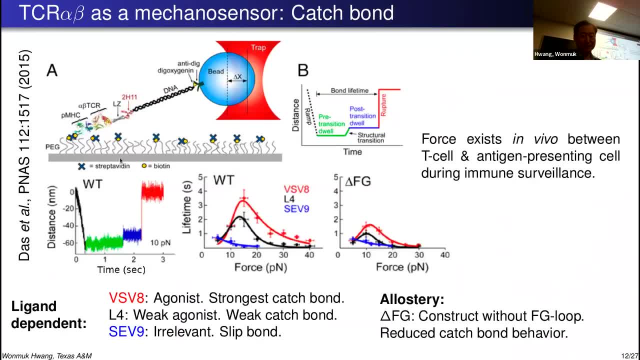 for that right, Because if the force that's meant to be the weakest force, Yeah, Yeah, Yeah. so without force, these are almost indistinguishable, And this 10 to 20 piconewton force is actually. 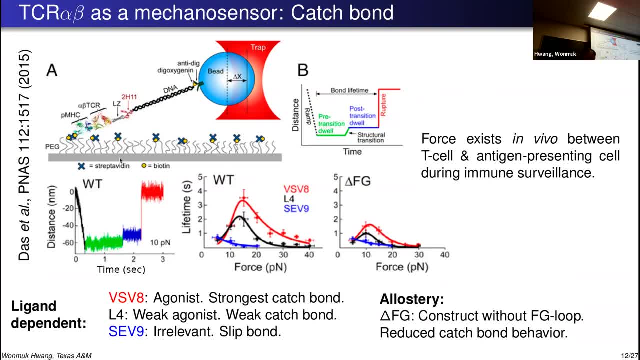 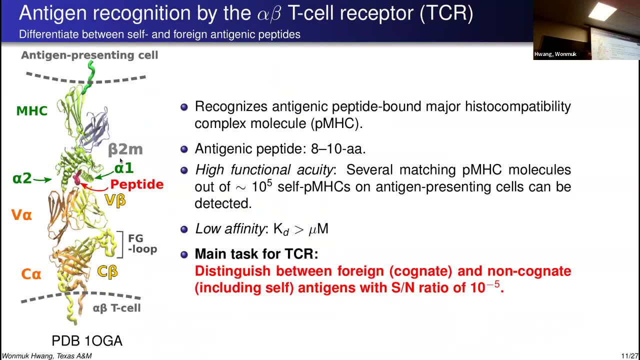 the physiological level of force. Yeah, I mean, when we do this immune surveillance, T cell moves relative to the antigen presence. They move around. So when they make transient context, yeah, they move on. that's the pulling force. Yeah, that has been measured: 10 to 15.. 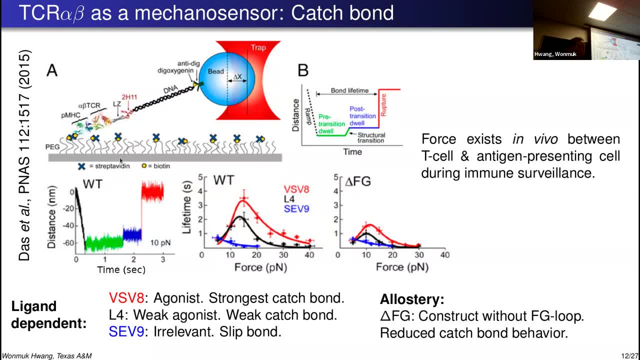 But I just so, the fact that the fact that in the presence of force- which I understand is physiologically problematic, right Mm-hmm- Is when this thing works best, I think, necessitates that the linkage that that. 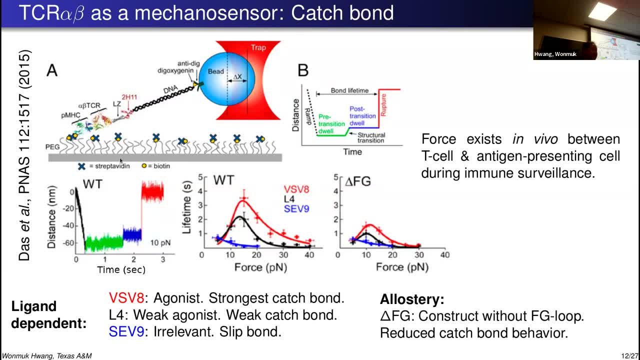 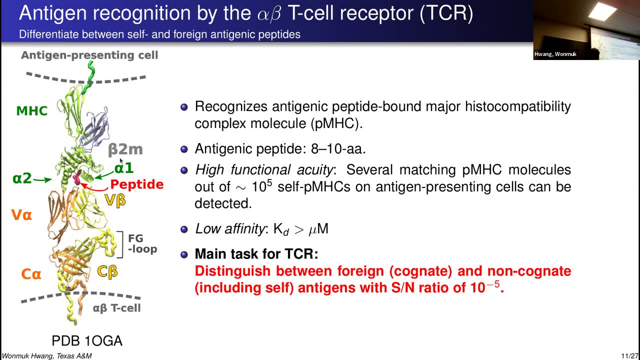 binding, intermolecular binding, otherwise it would in nature, the molecule itself before Right. Oh yeah, that's one aspect, And the other aspects I mean, yeah, if they are strong, then what happens is, I mean, these T cell receptors are sort of randomly generated. 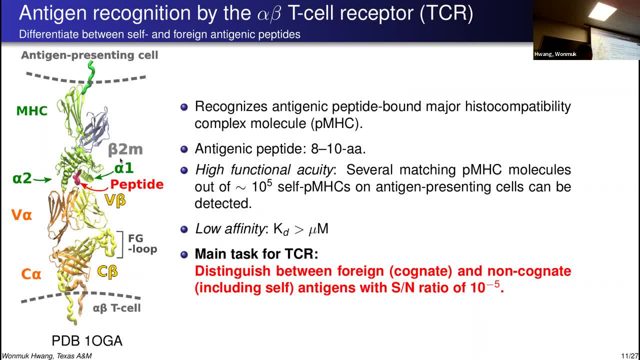 Yeah, if they are strong, then what happens is: I mean, these T cell receptors are sort of randomly generated. Yeah, if they are strong, then what happens is: I mean, these T cell receptors are sort of randomly generated in our body because we don't know what to expect. So we have these random T cell receptors. 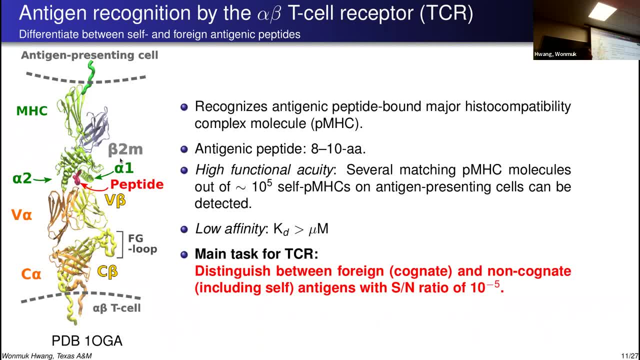 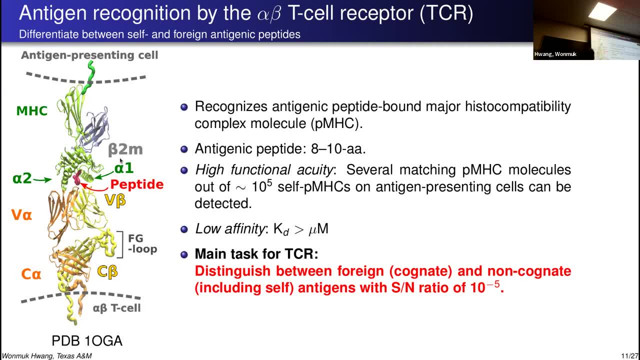 So positive selection means the T cell receptor has to have some basal binding strength. So those are initially selected, Then among them they are screened for negative selection. If they are too strong interacting they are deleted. So you only have a real, like range of interactions. strength that's, weak That's. 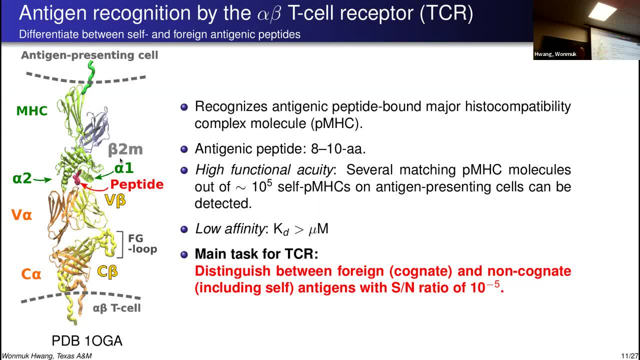 I think how they select weaker than the stronger. binding Yeah again if they are too strong, I mean yeah, even if they may not unfold. it's going to be difficult, Just like the kinesin walking with the wet feet. 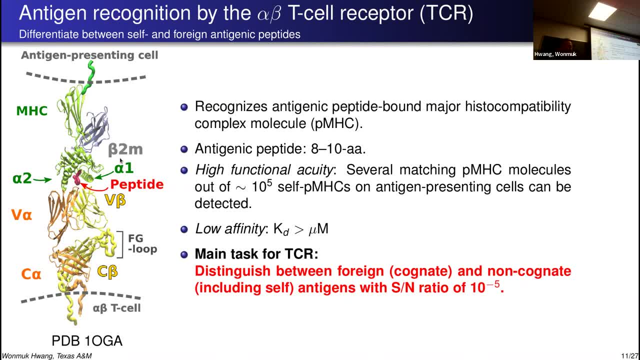 Just to know that. you know, Marcia is our expert on, let's say, optical tweezers and torturing the molecules, So I'm sure you have a lot to talk about Any other. Yeah, sure, David. So the fact that you mentioned this several times, because the feet are wet, 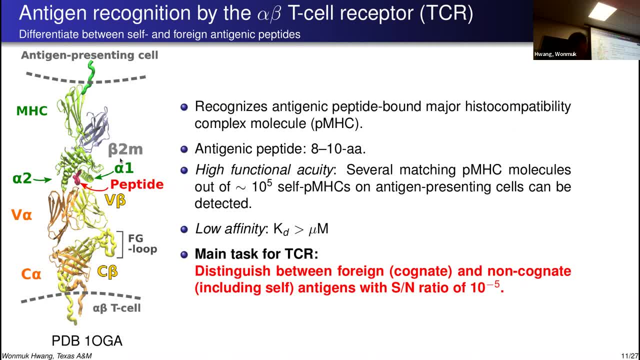 yeah, why is the wet important? Well, because when they make detach from the surface, if they are dry, that means it's mostly like hydrophobic interaction- then it'll be difficult to detach. So the binding has to be something that can be easily broken. 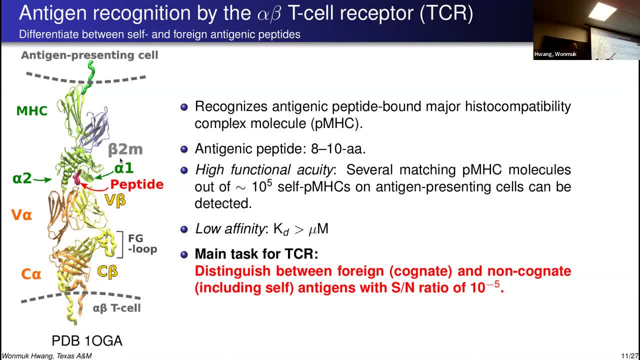 by some tiny conformational change And it's better to have water interface and hydrated interface. So if something is wrong then they can easily detach. So the water is electrostatic free. Yeah, if they are a little farther away When they are in the hydrated case. 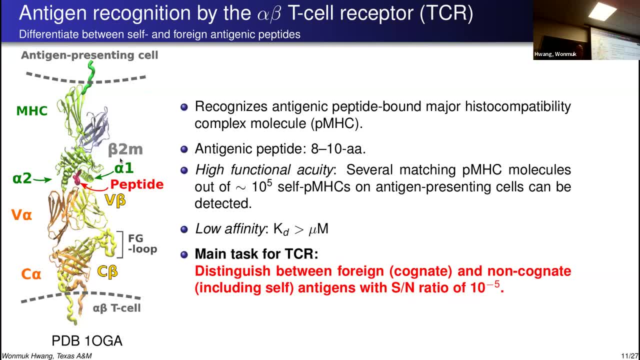 the distance is, yeah, within the divided length, So the screening will be difficult in that bound state. But when they are like this, then yes, the screening can play a role And actually you can control the speed or the run length by changing the source concentration. 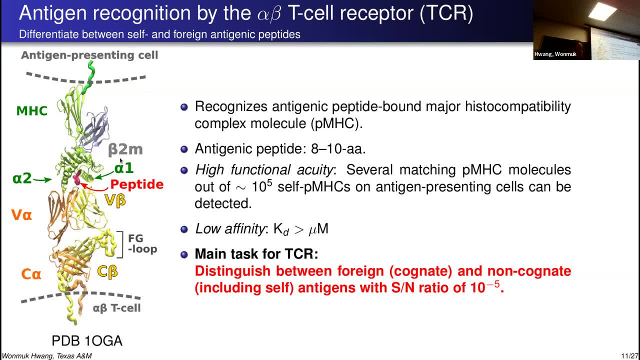 Okay, Yeah, And since you have this slide right, I think you mentioned that you know, for different organisms, right? so the lens of that p-loop, Yeah, Is very different, right, Yeah? So you know, have you, you know, explored that and you know, have that hypothesis or-. 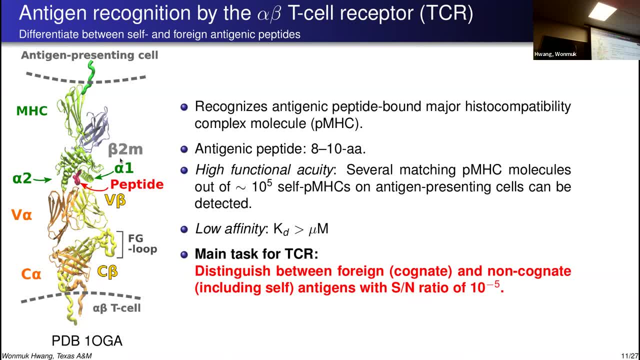 Not yet. We mean yeah, I mean first understanding human or a mamellion is challenging here. Yeah, Yeah, We mean yeah, I mean Yeah, Yeah up right now. so if you have a very good understanding then we may move to other organisms. 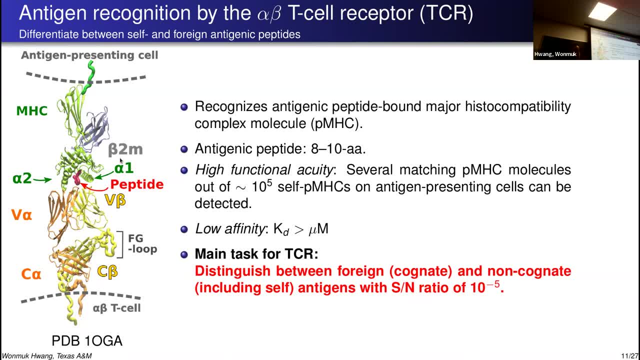 uh, that's one thing, and the other thing is availability of experimental data. people mostly work on mice, or you know. that makes sense. did i actually understand you correctly? so you said vertebrates, but you said vertebrates with jaws, yeah, jaws. so what the hell is the? 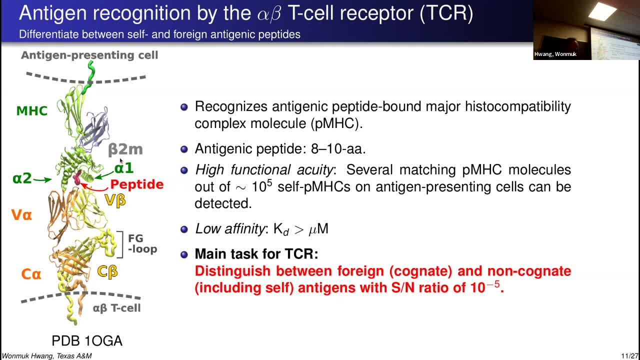 connection between having a jaw and doing this and not having a jaw and not doing it. so i- yeah, i had the exactly the same question, so i pondered about that. so jaw vertebrates i guess have more, i mean diverse range of food to eat, so they are exposed more organisms. so this prop. 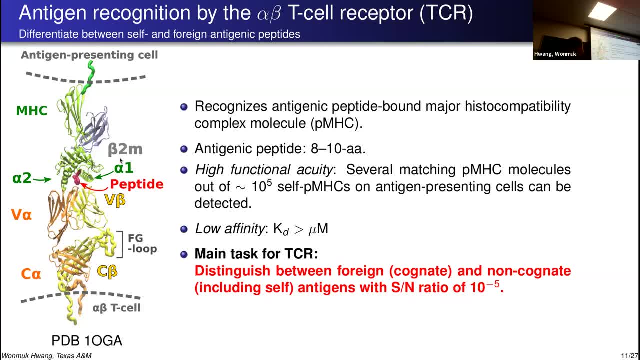 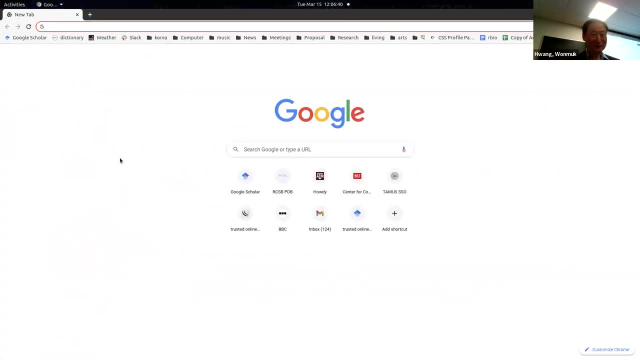 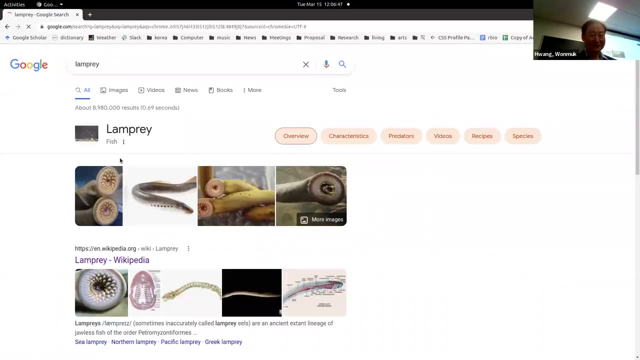 that's my guess. yeah, so, which is why they need to have, like, more advanced receptors. and then my the other question was then: are there vertebrates without jaws? and i hope the internet works, yes, so, yeah, they're this lampreys, that looks scary, yeah, really. yeah, it looks like uh from. 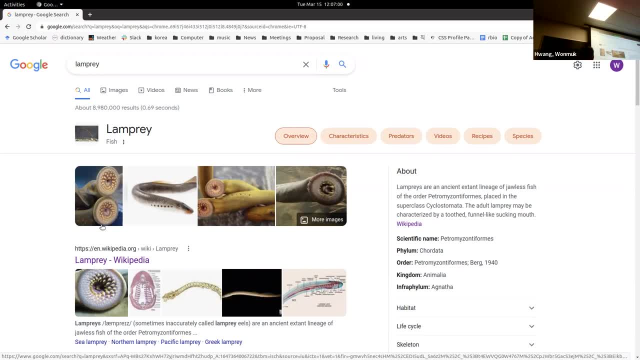 this alien alien, yeah, so they have, oh yeah, mouse without jaw, but they have vertebrates and like the way that they have, uh, it's not exactly like they just get fined. uh, they have tietalt right, so, like, the projections of the jaw are actually very high, so they have. 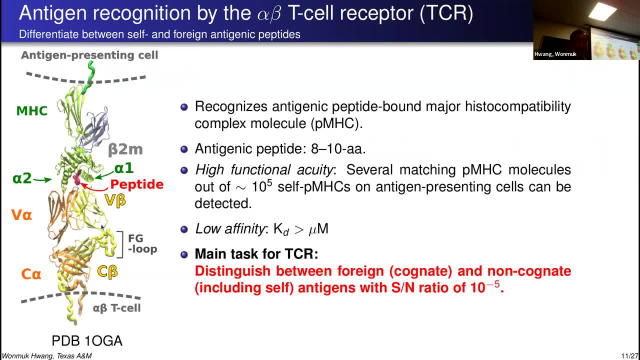 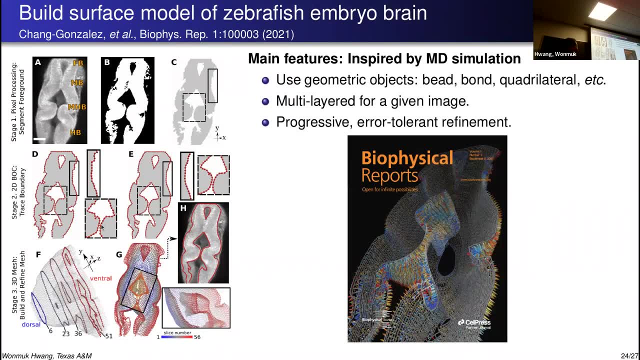 no activator and if they have real intelligence. that was quite interesting and casey. my my only question is: are there any studies? i don't think there are any examples where so many people did scientific rapid indications. what? where are the parameters right? so what was needed to develop those parameters to make the 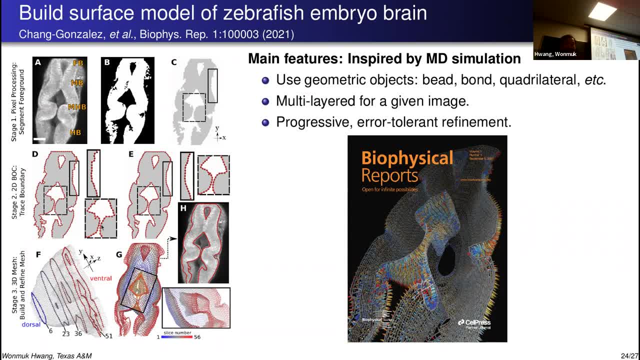 refinement work. yeah, i mean. first of all, there is no force field here, it's just a static structure. the idea was to represent this in terms of b's and bonds and so on. right, so yeah, if you, yeah, read about this image processing literature. almost all of them work at the level of pixels. 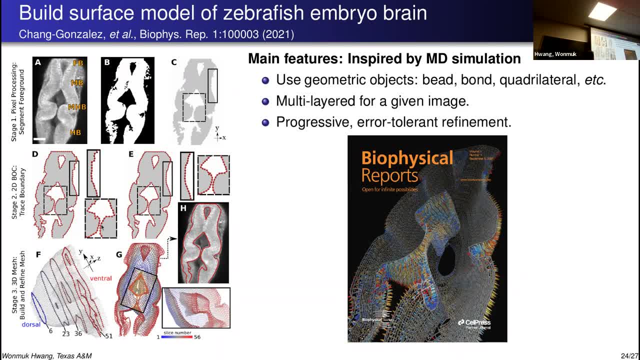 but each pixel doesn't carry information about this structure, so you need some sort of course screen picture which kind of base inspired how to use this like geometric object assignment. so these here locally represent some uh features of a group of pixels, like nine pictures, and so yeah, then yeah, connectivity and so on and so forth. 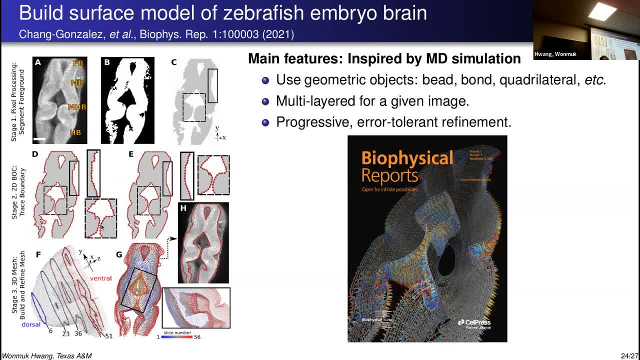 and yeah, this output is written, actually as a charm, psf and coordinate files, so then you can visualize using pmd or other right. but i guess what i'm curious about is: i mean, there's representation, right, yeah, but then usually, whatever computation you do, yeah, you have to like. 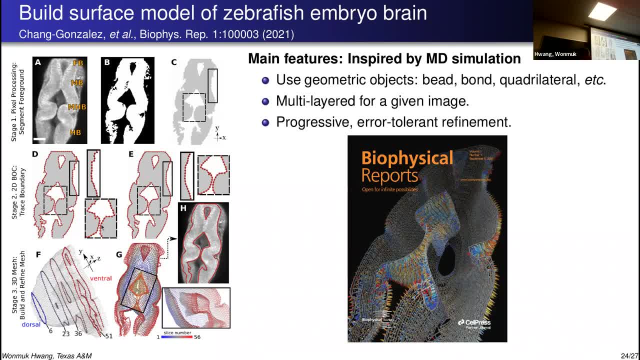 either optimize something or maximize something, right, and so what? what? what is being? yeah, what is the cost function? yeah, so those are, yeah, they're kind of refinement. so if you just do this, uh, beta chain assignment on a single image, it's rough, but you have these layers of. 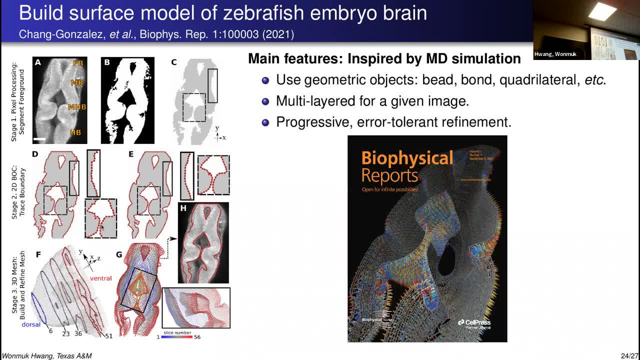 your chains. then if you apply, say, the continuity of the surface, because the real structure, the surface, won't be this rough. so if you apply the continuity, then it becomes smoother. so it's it's kind of like applying energy minimization locally on the surface. yeah, that's one. 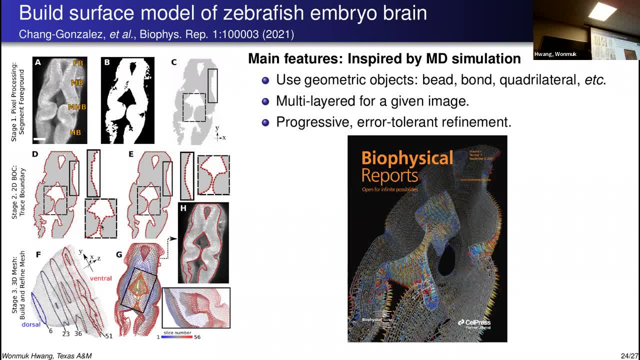 look at it and yeah, the other way is speed, because this image analysis takes a lot of time if you just use Java or Python or, yeah, MATLAB. But if you write in a C++ and make it actually the comment-driven, it can be much faster. 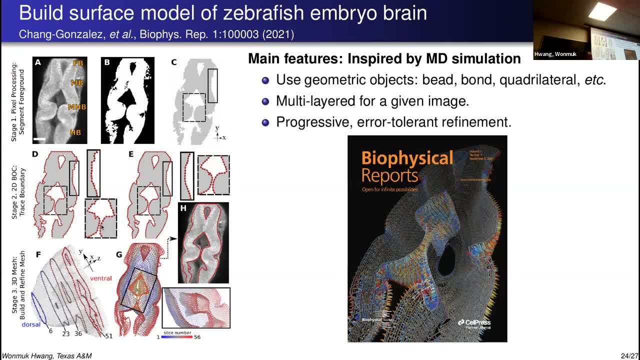 But the follow up on this question, like the parameters of the spring constants for the bonds and the various other things that influence the shape of the net right Or, if you want to, How robust are the structures you predict for this or the structures you visualize for this? 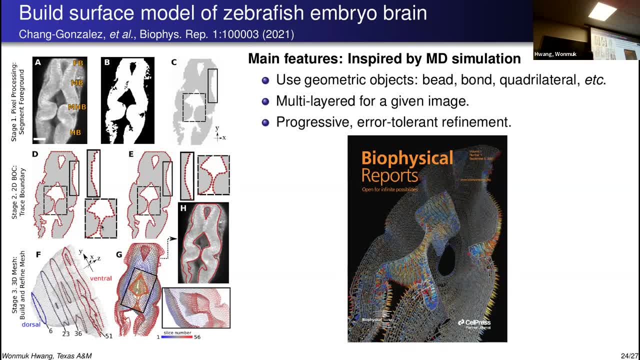 the choice of those types of parameters. Yeah, so those parameters you have to. I mean, right now it's kind of semi-manual tuning So you choose how many pixels you want to use for assigning a BDL. I mean that's usually dependent. 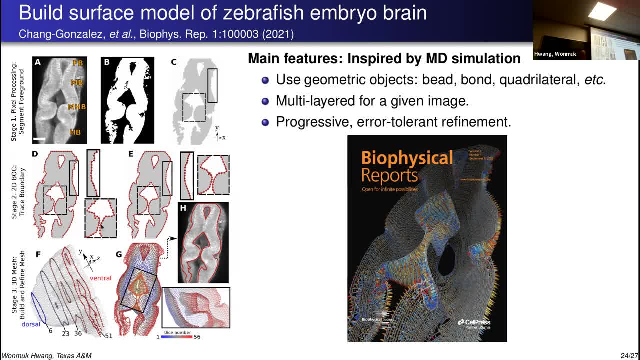 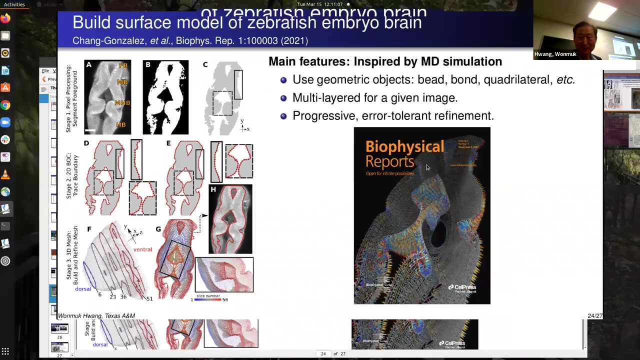 I mean determined by the length scale of this BDL, Usually the range of length and the length of the features. So over one range of length does this change significantly? that gives the range of say, oh, i mean, there are people online. i don't think so. any questions from online people? yeah, our virtue. 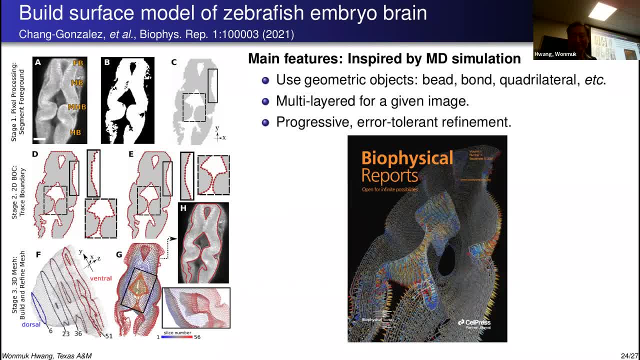 yeah, hi, john, you have any questions? the problem is like: oh, i can't hear you. yeah, that's right, somehow we can't. can you hear us? i can, i can hear you. yeah, they can, okay, but we can, we can't hear you. oh, yeah, the problem is: yeah, my laptop doesn't. there's a sound from here, i mean: 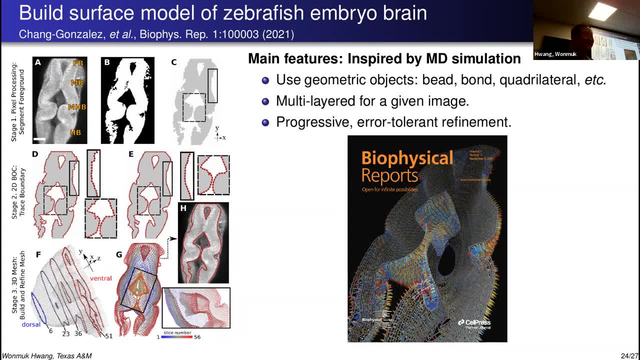 yeah, if you have questions you can type into the chat box. my sound might work. can you give me the link, the link, the passcode, oh, uh, here. oh, there is that. 960, all right, oh, 1037, nine, now anything that works. just a minute, and the password is. 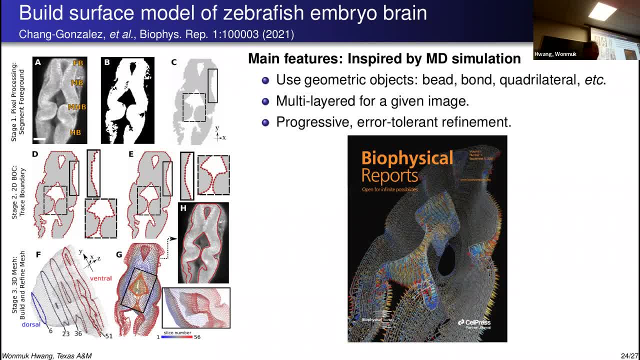 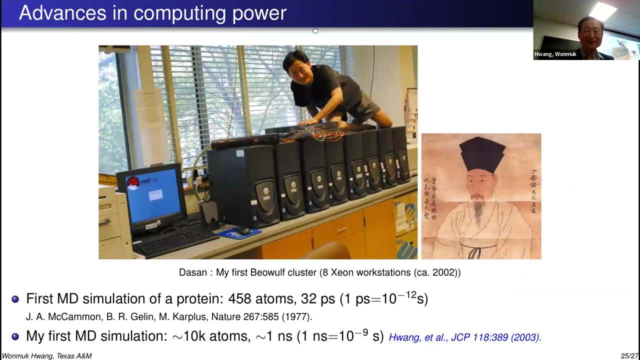 oh nine. two, oh two, three continue. okay, got it. wi-fi recording in progress. okay, too many devices. yeah uh, john, john, do you have a question? is john still there? john is still there. can you hear us, john? Oh yeah, Say something. Can you hear me? 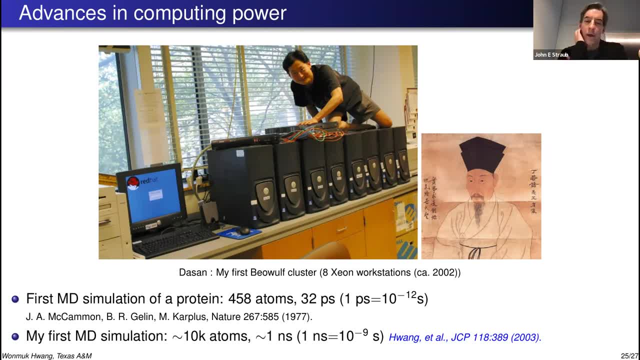 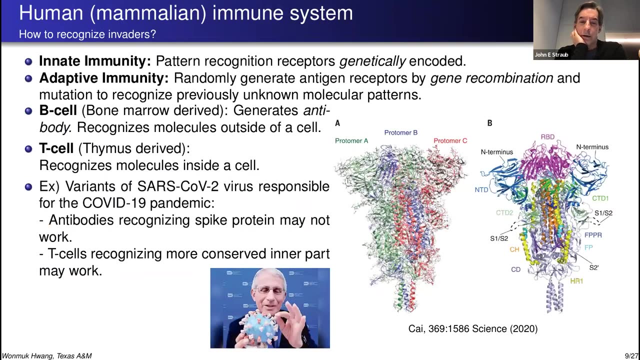 Yes, we can. Okay, I was just typing a question, So thanks for a great seminar. I mean, going back to the beginning, we were talking about DNA organization and chromosomes and so on, And I was wondering if you've seen any sort of out of equilibrium dynamics or glassy sort. 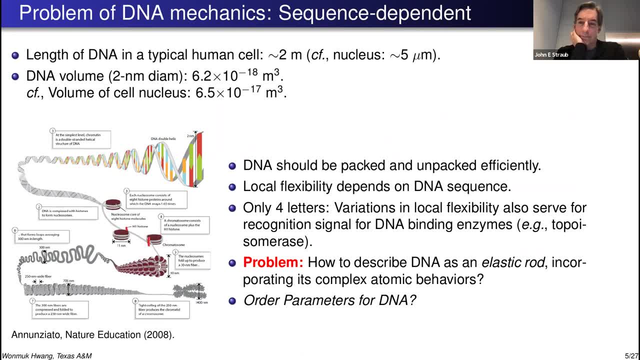 of behavior in any of those systems. Yeah, you know, DNA can unfold and so on, And our model is limited within the linear elastic regime. So our model right now doesn't address those transitions and glassy behavior. And glassy behaviors, I think, are more for the aggregate or the assembly of DNAs rather 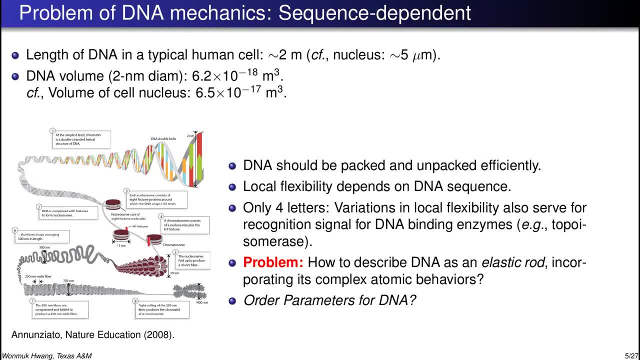 than individual base pairs. Yeah, what are your thoughts on those more sort of large scale, ultra coarse-grained models of DNA? Well, actually we compared our model with West's DNA. I think from Oxford they had this coarse-grained model. 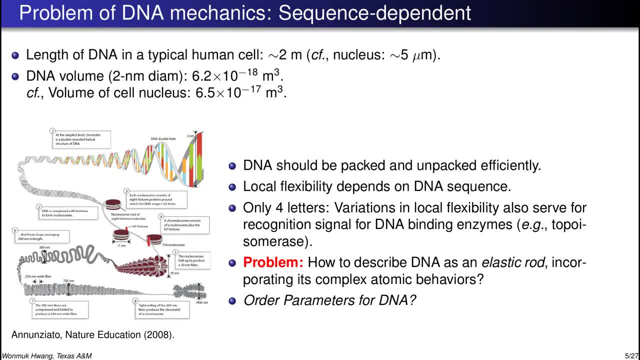 And in terms of capturing the mechanical behavior and sequence-dependent, our model works well Because their West's DNA was more for the transition And I don't think they parameterize their DNA like the elastic properties based on the sequence-dependent way. So by design their model is, I mean, yeah. 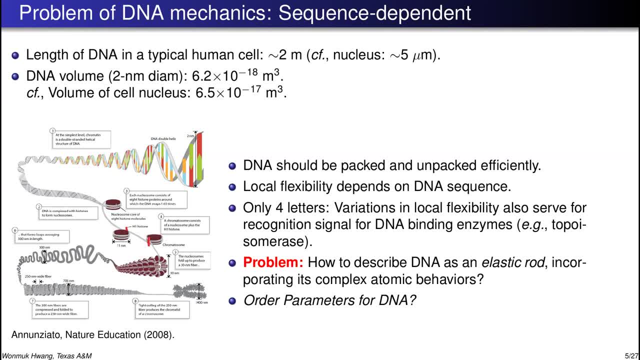 Their model is focused on something else than what we studied. Yeah, So in terms of DNA looping and persistence lengths people measure, our model gets the numbers sort of better. So you're more of a proponent of sort of bottom-up coarse-graining, starting with more microscopic. 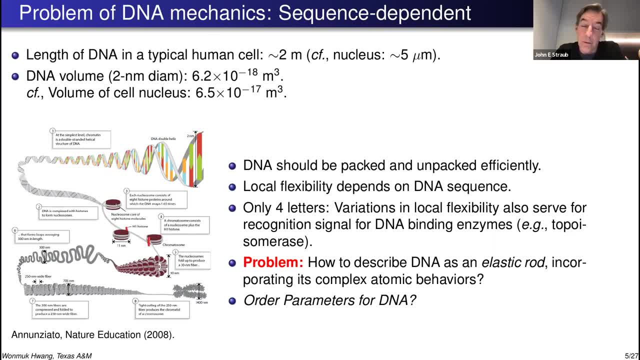 models, Yeah, And coarse-graining rather than the top-down, for even Even for these types of systems, Yeah, I would say so Because I think coarse-graining has to be based on certain properties that you are interested. So if you do top-down, sometimes if the behavior is very regular, then you can capture the 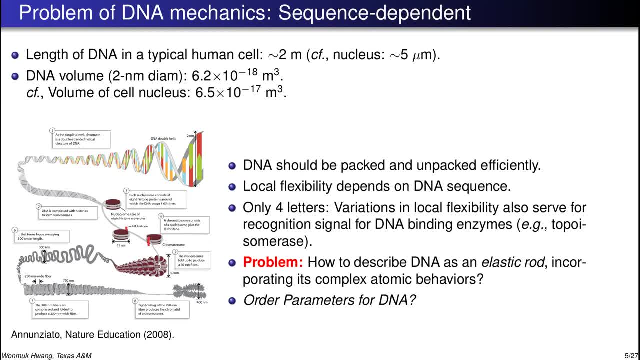 underlying dynamics from top-down approach. But for a lot of biomolecules, you know, Yeah, They are very finicky, So you have to understand their atomistic behavior first before building the coarse-grained model. And yeah, in that lines of thought, I am not very fond of generic coarse-grained force. 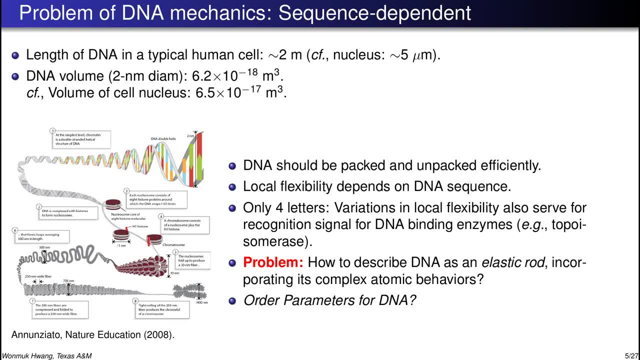 field in, Yeah, Such as martini. Okay, They have. Yeah, I know that you use martini, but, Yeah, Yeah, It has its uses. But, Yeah, Yeah, Yeah, Let's. I have had to say a little bit about these robustdaughter for information. 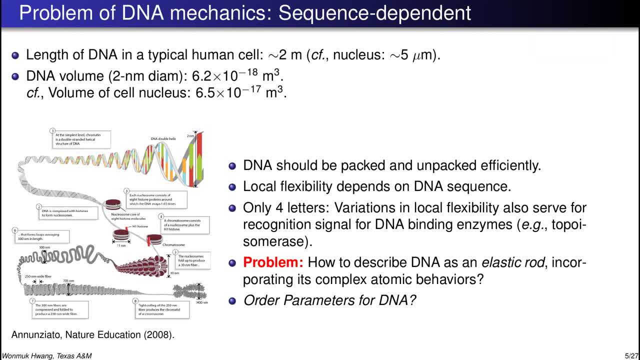 Yeah, It was a. uh, So you can, It was just a very good. No need to speak too much. Yeah, it was, there was one that was quite good. but if you want to study like motility of kinetine, kinetecin. 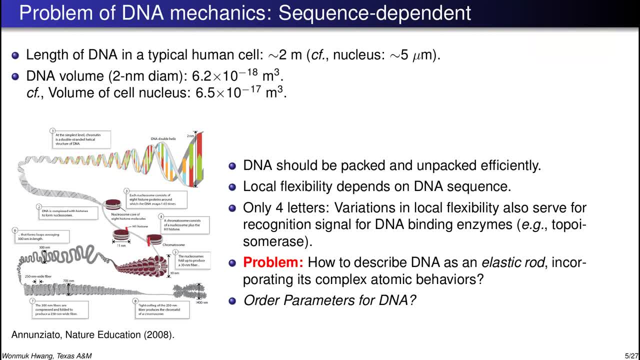 or aggregation of certain amyloidogenic proteins and so on. yeah, it's better to, yeah, put or system-dependent parameters in your model. That way you can capture the behavior better. I think, Yeah, I mean, I think it's a very interesting question. 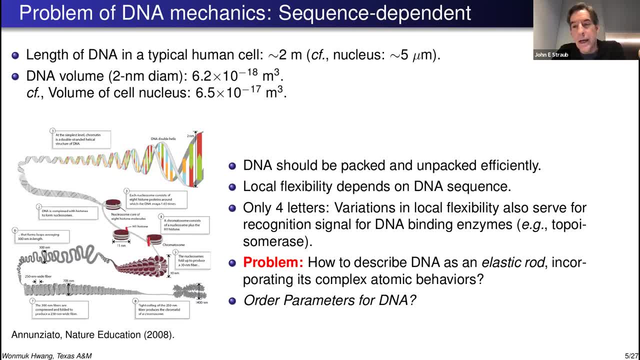 It probably depends a little bit on the question you're asking, right, What type of model? Yeah, Exactly, reach that. But I know there are people doing very good work, like on RNA, Giovanni Busi- that are more proponents of a top-down model. Greg Voth, of course, is a proponent of bottom-up. 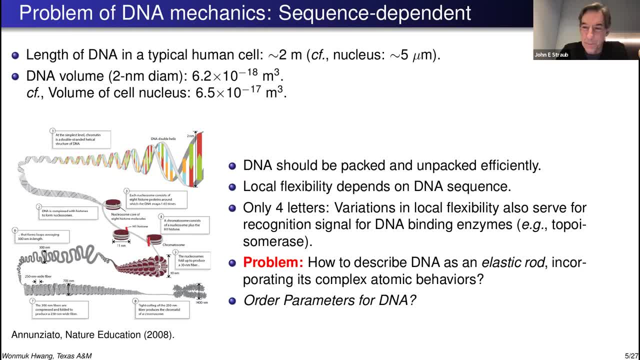 and so, anyway, probably depends on the system. Yeah, And besides, I think bottom-up is more time-consuming, in a sense, than top-down Is more what, sorry, Time-consuming to develop. Yeah, Yeah, Good, thank you, Thank you. 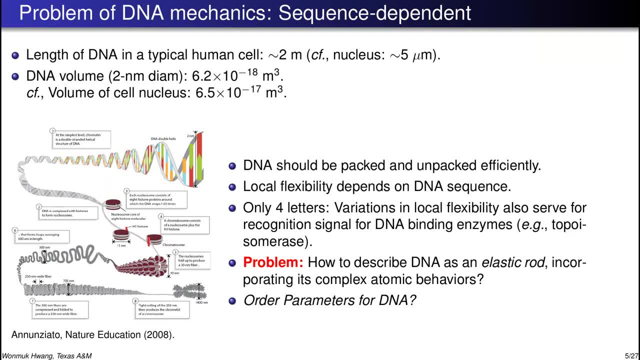 Thanks, John. Any further questions? Okay, Let's thank Juanma for a really great talk. Thank you very much, David. are you using quantum teleportation to send me that lunch? We're working on that, John. We're working on that. 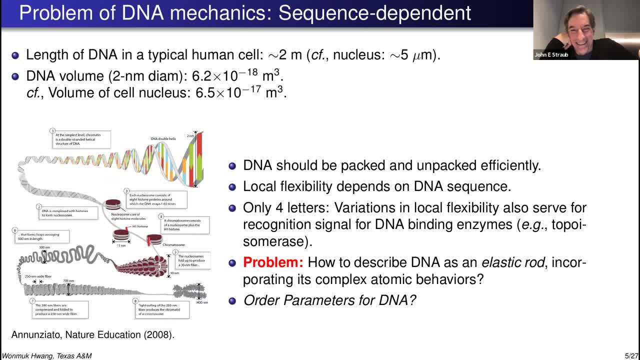 Not quite there yet, Want to try it out. We have a coarse-grained version of one. It was bottom-up though. All right, Have fun, John, Take care. Good to see you, Thanks, Bye-bye, Bye.